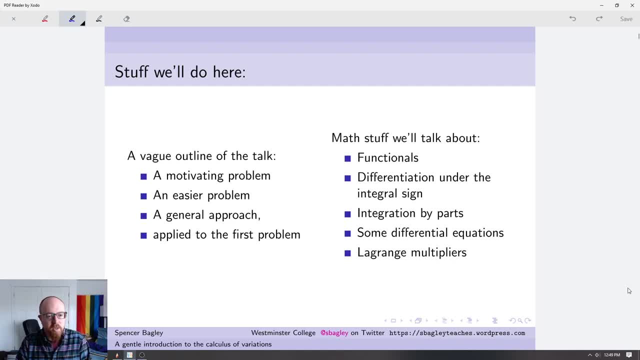 one that's interesting, but it's also going to be like too hard for us immediately, so we're going to think about an easier problem instead. That will help us decide what the general approach is, and then we'll go back and apply that to the motivating problem. A bunch of fun. 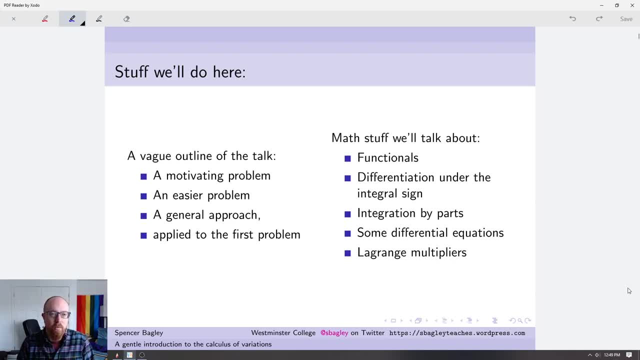 math stuff is going to happen here. We're going to talk about functionals, We're going to talk about differentiation under the integral sign. We're going to do integration by parts a couple of times A very small amount of differential equations, and then Lagrange multipliers make a surprising 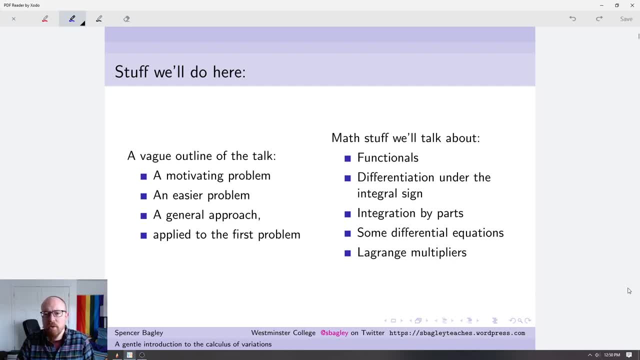 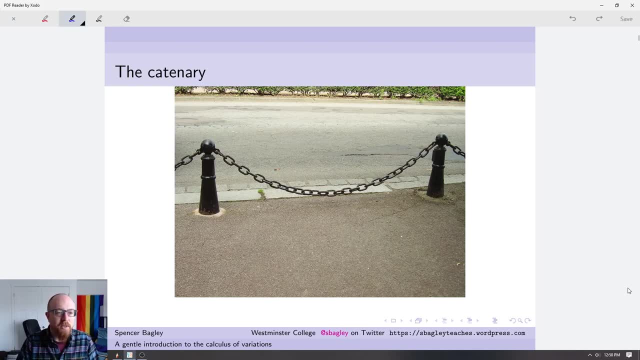 appearance at the end of the talk. Okay, so here is the motivating problem, and it's called the catenary problem. So catena is Latin for chain, and so the question here is like: what is the shape that a hanging chain takes Specifically? can you write it down as a mathematical function? 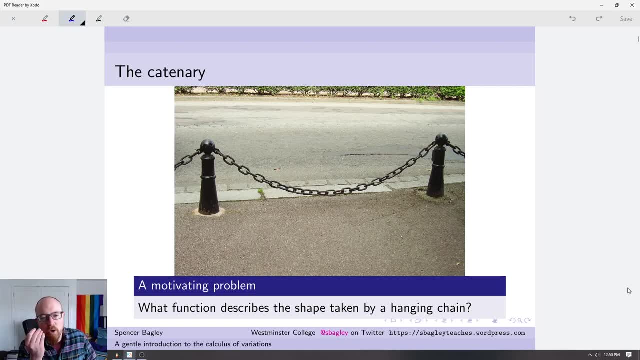 If you look at this, you could sort of say, hmm, maybe it's an arc of a circle, maybe it is an arc of a parabola, maybe it's something else, I don't know, And so that's sort of the interesting problem that we're going to try to answer at the end of this talk. 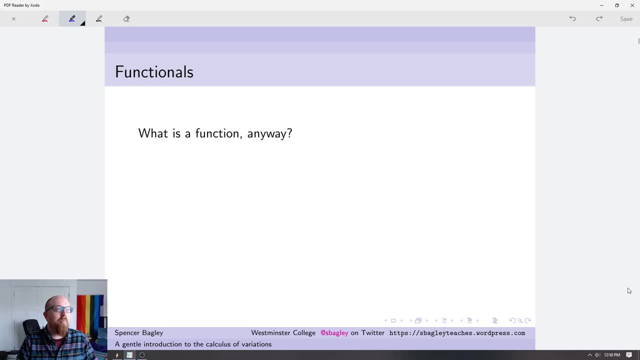 But that's clearly way too hard for now. So let's back up and we'll think about an easier problem, and we're going to think about it in terms of functionals. Now, what is a functional? It's a kind of function. Okay, what is a function? A function is some kind of rule that associates 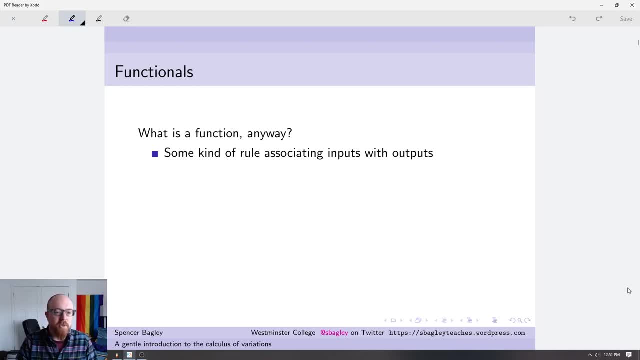 inputs with outputs, Most of the time with the functions that we're used to dealing with. we think of functions as maps from the real numbers to the real numbers. So we have one real number input and we're associating with one real number output. Okay well, 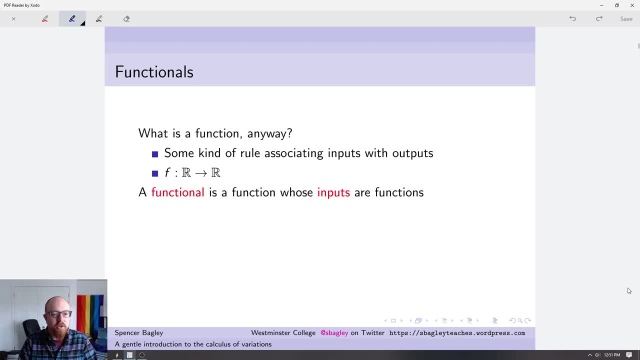 a functional is just a function. who eats functions and tells you numbers? So the inputs are functions and the outputs are numbers. So you might write it like this: The letter J, capital J, is traditional for some reason. Don't ask me why. We're probably going to think about. 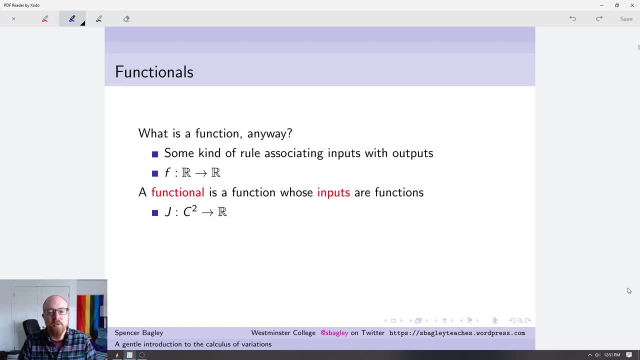 functionals on C2, which is the space of twice continuously differentiable functions. That's smooth enough for our purposes. There are, of course, other function spaces that we could play with, but that's as spicy as we need to get. By the way, if I were naming this subject, I would 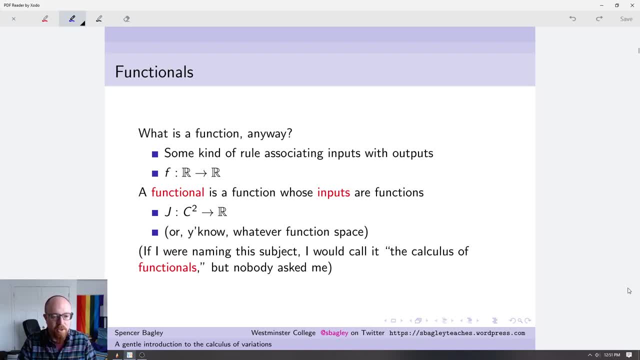 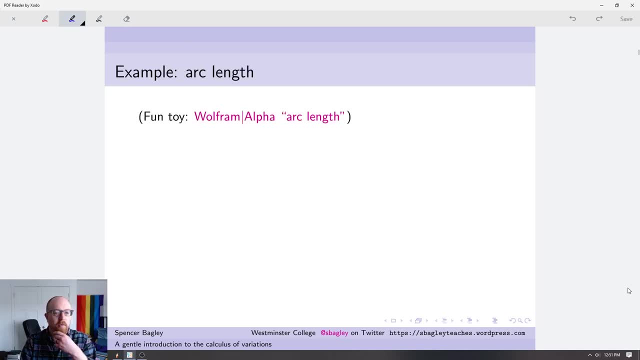 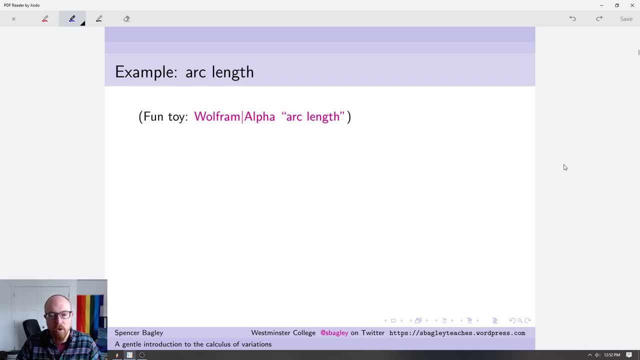 If you click on this link it will take you to the Wolfram Alpha page for arc length. Or if you just go to Wolfram Alpha and type in arc length, you will get a cool little calculator. Let me show you what that looks like. 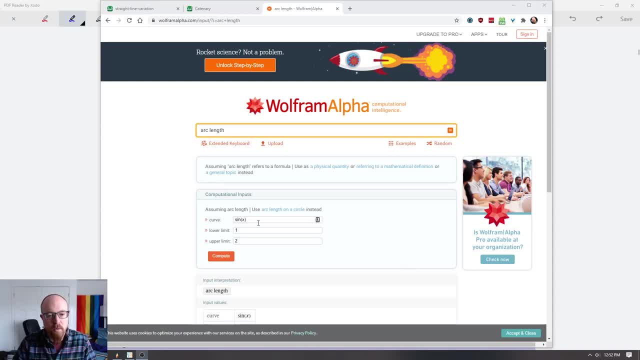 Okay, here's the Wolfram Alpha page for arc length And you can see what's going on is we tell it a particular curve, a particular function, and we tell it the X value that we want to start at and the X value that we want to end at. 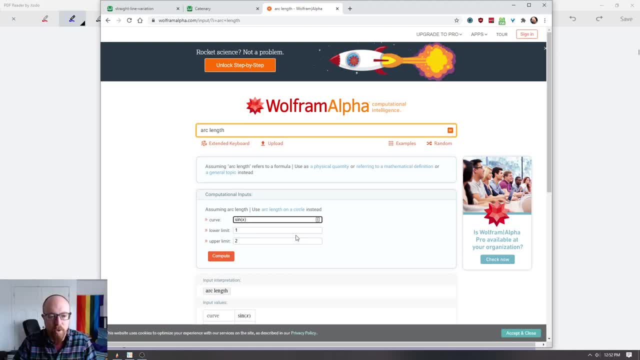 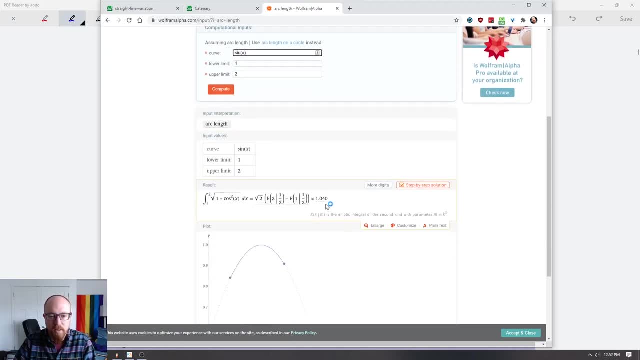 And it calculates the arc length of that function between those two points. All right, so the sort of default settings on Wolfram Alpha are sine of X from one to two and it does whatever it does and it tells us that the answer is 1.04,. 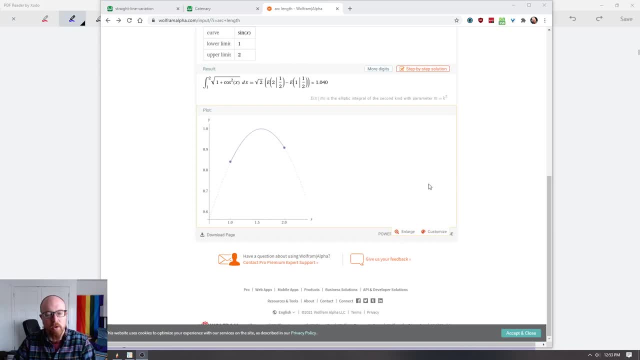 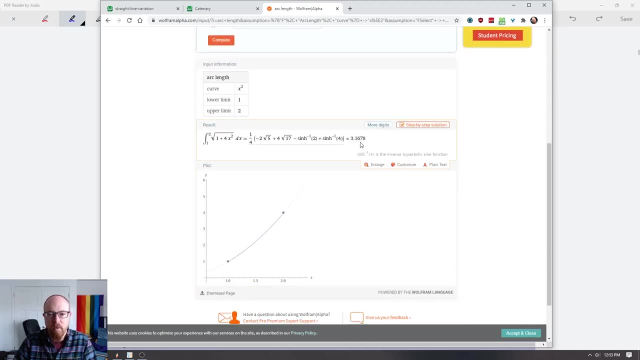 and it draws us a nice little picture. Okay, we could throw in some other function here, like, I don't know, X squared, That's a fine one, And it again does whatever it does and it tells us some number: 3.16,. 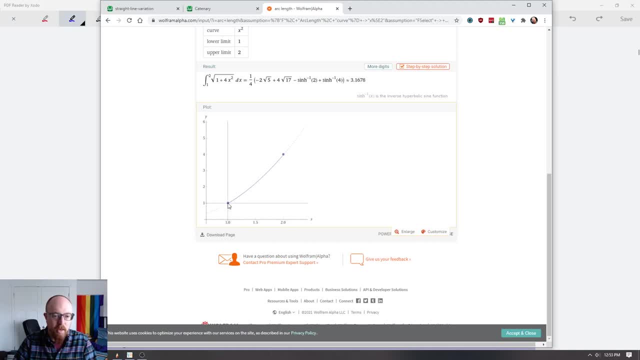 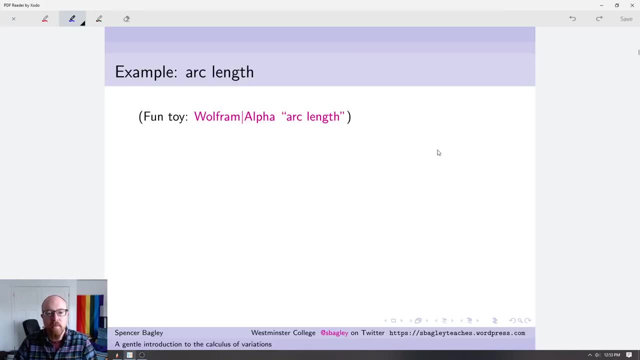 and you can see this picture. the arc length between X equals one and X equals two. It's the length of this piece of line. Okay, cool. So my point with this is like, legitimately, this is a function whose inputs are functions, right? 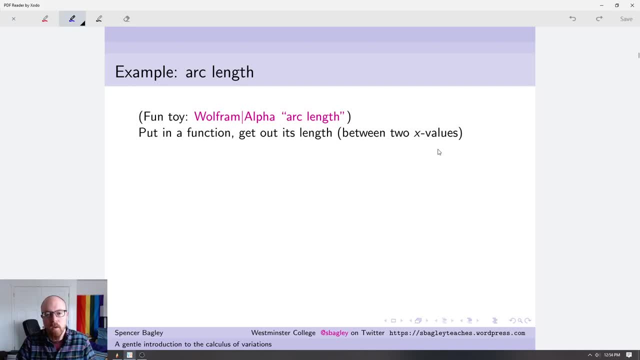 If I put in a function, I get out its length between two X values. Let's see if we can write down what Wolfram Alpha is actually doing in the background here. And to do that we're going to do a little calculus. 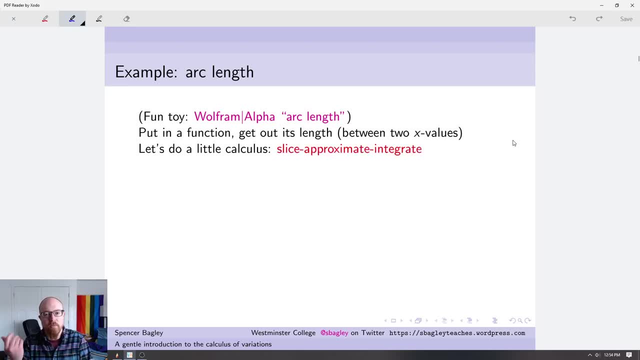 We're going to slice, approximate integrate, which I like to think of as like the fundamental paradigm of integral calculus. So here's some arc and I'm going to look at a little piece of it and I'm going to approximate the length on this purple curve. 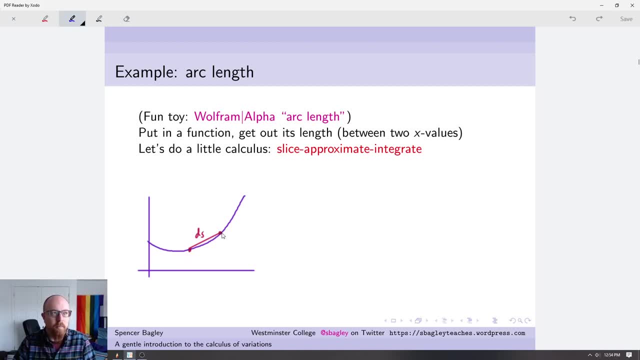 by a straight line which I'm going to call ds. I don't know why we always call lengths s probably German or something whatever. This is not the right answer. clearly, The purple line is a little bit longer because it bends away from ds. 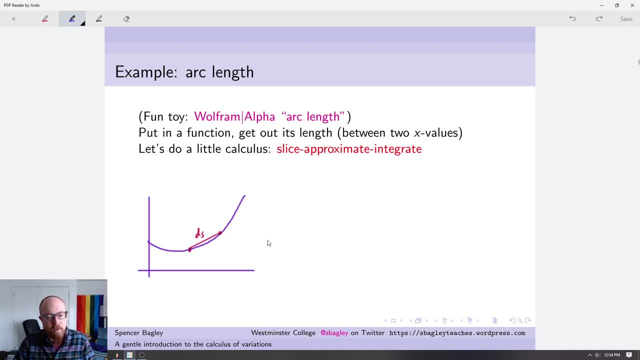 but it's a pretty good approximate right And, what's more, it's easy to calculate. Specifically, it's the hypotenuse of a right triangle with sides that I can think of as dx and dy, And so that means that ds squared. 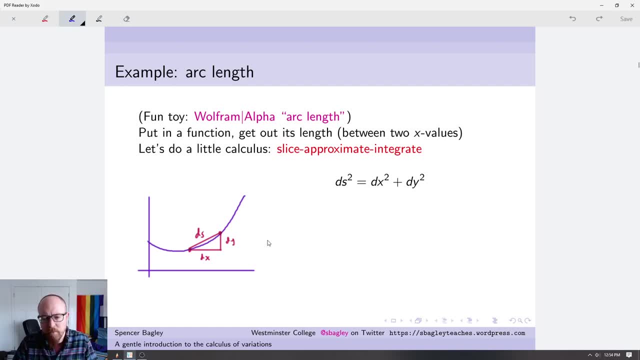 ought to be dx squared plus dy squared. I'm going to play a fun trick and factor out a dx squared like this, because then I can recognize this as: oh look, that's dy dx all squared, which is the derivative. I can take the square root to get ds by itself. 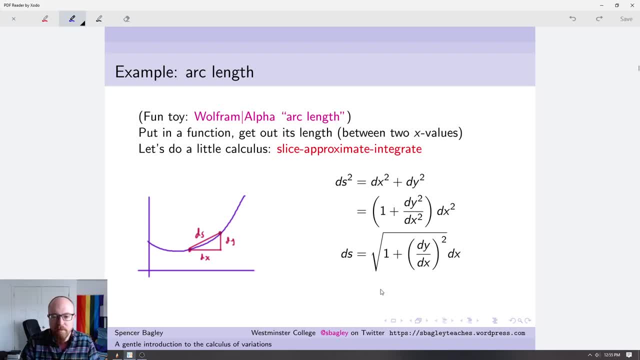 I'm not going to worry about plus or minus, because it is a length and I want to think of it as positive, And so I end up with the following: We're going to see this a lot. that ds is the square root of one. 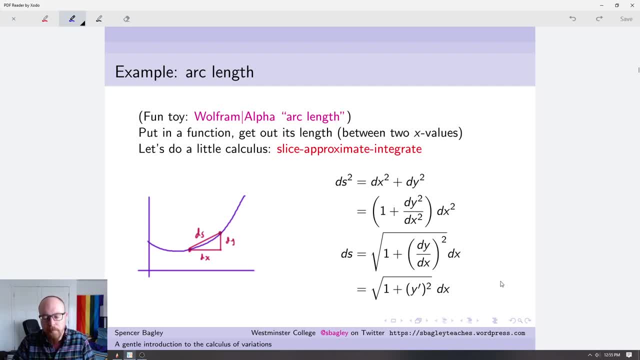 plus the derivative squared dx. So hold that thought. We'll see that multiple times. All right, now that we have figured out the length of a little chunk, we can add up a bunch of those and take the limit, and then we get an integral. 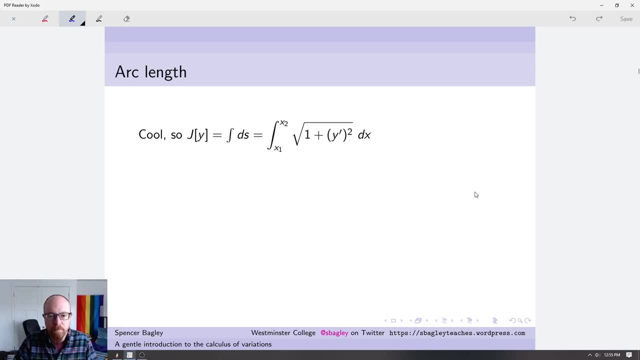 And here then is the formula for this: functional. Now you'll see, I'm writing it with brackets- That's also traditional- rather than parentheses to indicate that it's a functional rather than just a function. Nice little thing. Okay, notice here that this integrand is some function. 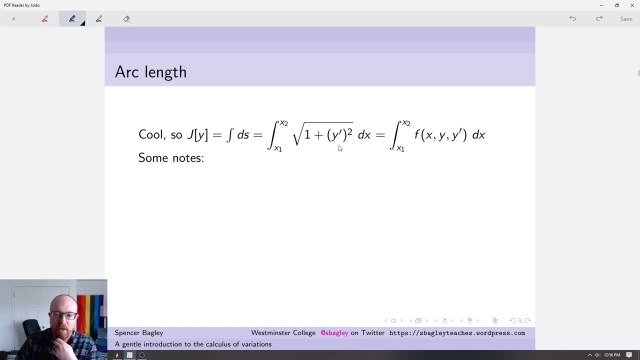 that involves it, for sure involves y prime. Maybe I could think of it as involving also x and y in later instances. Some notes here: most functionals that we care about end up being definite integrals because the slice integrate approximate paradigm is so useful. 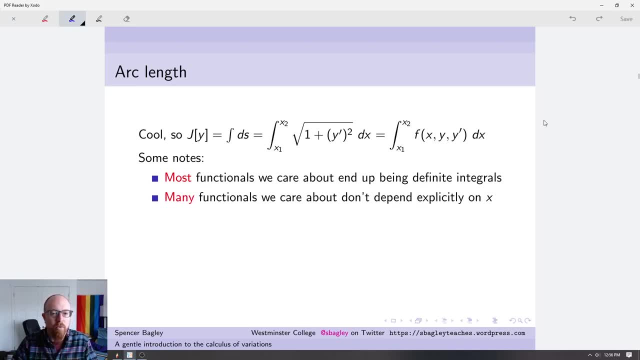 And many of the functionals that we care about, like the one that we have here, don't end up having x explicitly in them, because things are autonomous: I can shift them from side to side and nothing sort of bad happens. Okay, so then here is our easier problem. 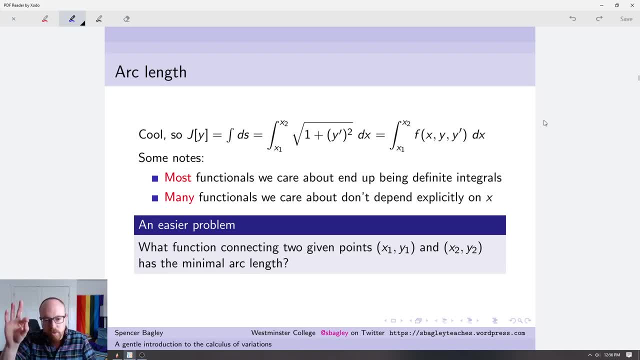 that we're going to solve. What function connecting two given points has the minimal arc length? Of course, the answer should be the straight line. I'm asking a question that I know the answer to, so that I can figure out the right way. 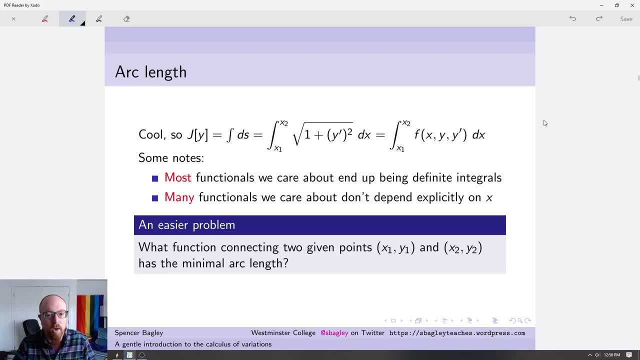 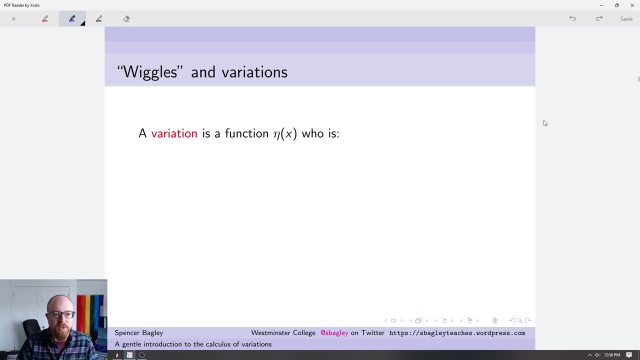 to figure out the right process to get the answer. Okay, we're going to need a little more technical tools here, and the tools that we're going to need I like to call them wiggles, and then variations. This is where the calculus of variations comes from. 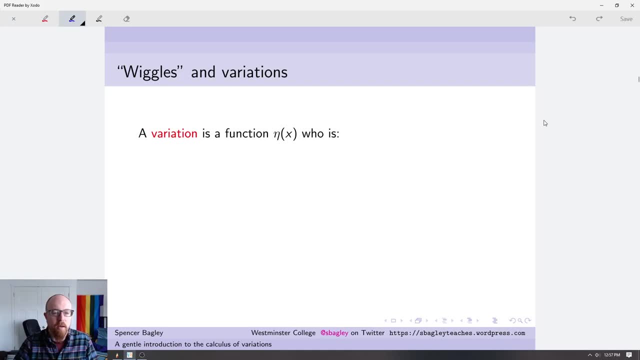 Okay, what is a variation? Variation is a function that I'm going to denote as eta of x, and it has a couple of interesting properties. First of all, it's not too wild. Maybe I want it to be piecewise c2.. 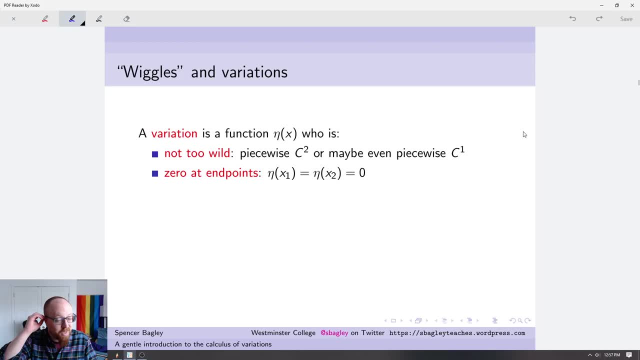 And then I also want it to be zero at the endpoints, and I'll tell you why in a second. Those are the endpoints of the definite integral, the region of integration that we're interested in, And then a wiggle is what I call. 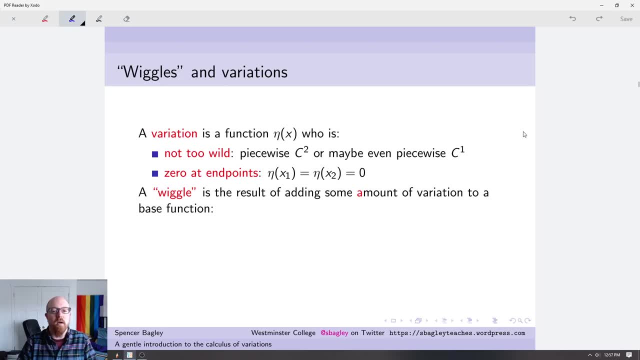 and this is not a standard term. this is what I call what we call a wiggle, What you get when you add some amount of variation to a base function. So I'm going to write it like this: A wiggle is our original y of x plus a times eta of x. 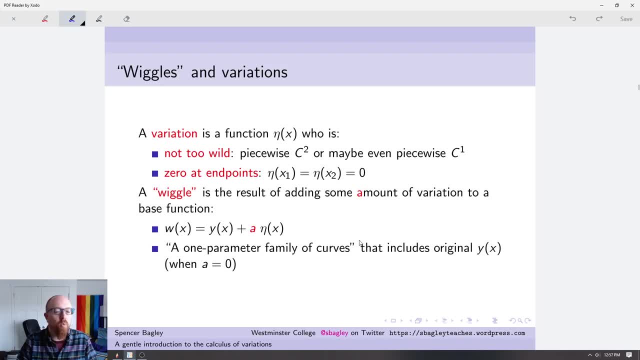 What is that a doing? It is giving us a one parameter family of curves that includes the original y of x, specifically when a equals zero, And so you can think of a as the amount of the variation that we are going to add to our original curve. 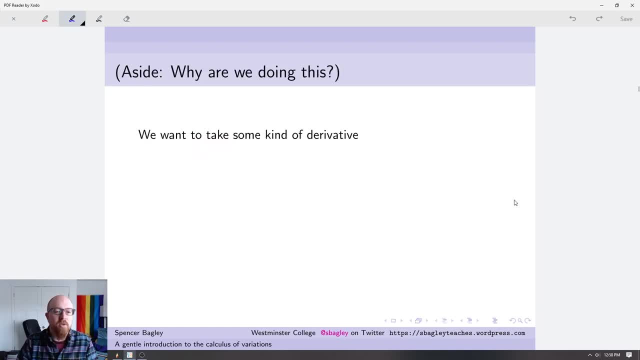 OK, What is really? why are we doing this? It's because we want to take some kind of derivative, because the right answer to our question is the one that minimizes or maximizes a functional, And derivatives are a good technical handle on extrema. 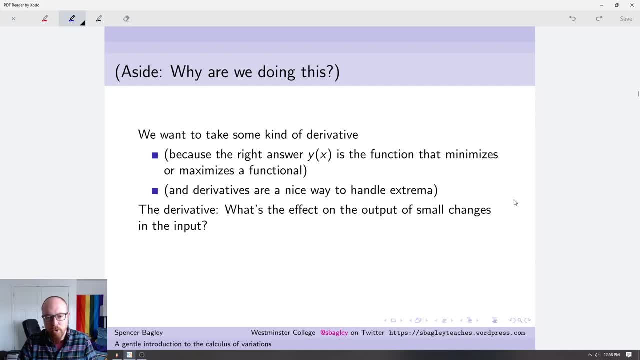 And so what a derivative asks is: what's the effect on the output of small changes in the input? And so, since our inputs here are now functions, I think that wiggles are good technical handle for us to deal with small changes to functions, small changes to our input. 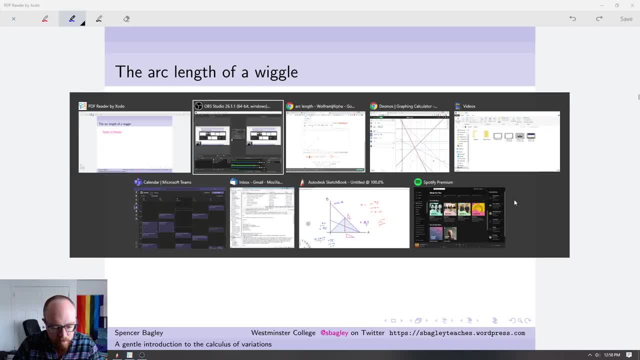 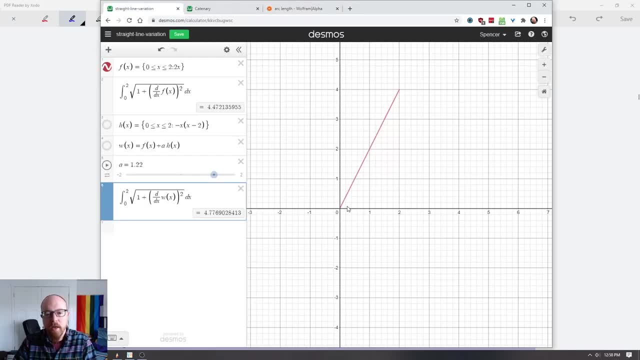 Okay, let's take a look at what this looks like. And I've got a Desmos pulled up here on one of my various pages, So here I have the straight line that connects the points 0, 0 and 2, 4.. And I've asked Desmos to calculate the arc length. It's this which is indeed the square. 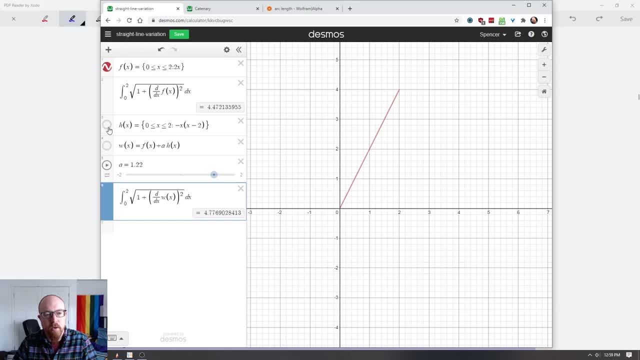 root of 20,, as we would expect. I also have here a variation, So you can see that this satisfies the criteria, that we have. It's 0 at the endpoints and it isn't too wild. And then here is a wiggle. 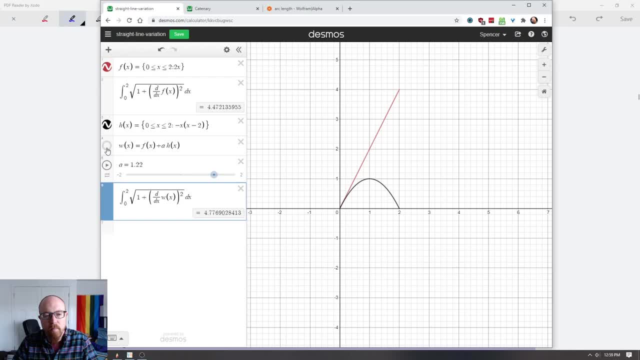 So what I'm doing is I'm taking this red thing and I'm wiggling it by a certain amount of the black thing And I can change the amount and you can see that right sort of perturbs the red function in just a little bit. 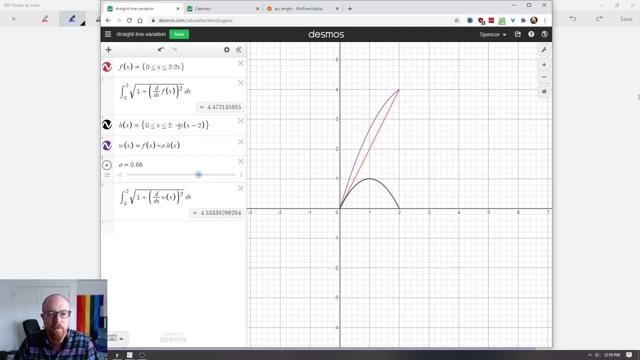 What's neat about this setup is that I could use different functions for h of x, Like: here's a wigglier one. How about the sine of 2 pi x? All right, well, so now you can really see that's really a wiggle, And I again have control over the amount of the wiggle And I could get. 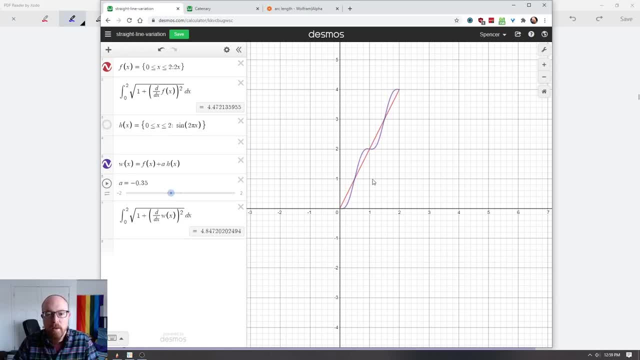 wigglier right. I could put any function in there that I want and still end up with some purple curve that connects the two points that it's supposed to connect. What's more, I have asked for the arc length of the wiggle And you can see it's in general going to be a little bit larger. 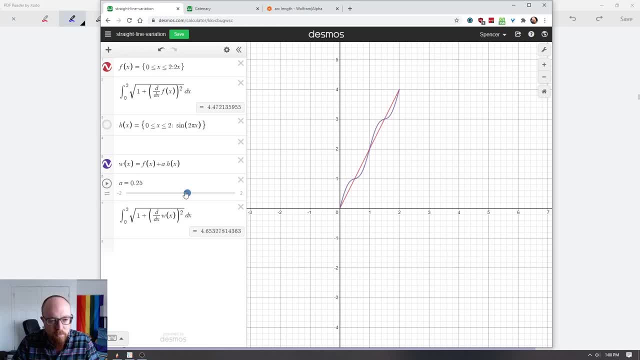 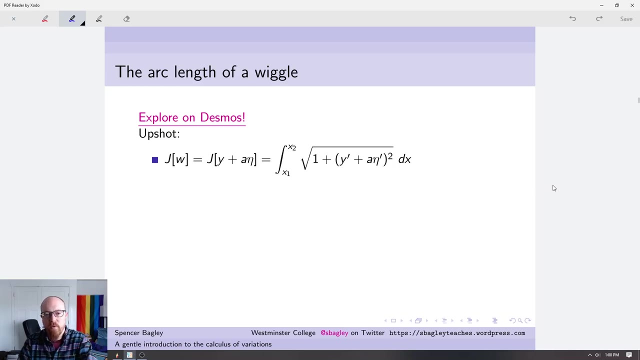 than the arc length of my minimal thing, unless, of course, a happens to be 0 and then they coincide. Okay, cool. So that's what's going on here, And here's my point. If I throw the wiggle into the functional, here's what I get, And truly, this is a function, a regular. 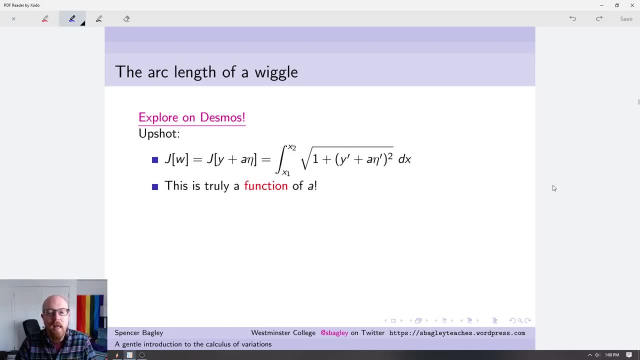 planal r to r function of a, of the amount of variation that is. And so if that's true, so I can write it literally as j as a function of a. And here is what it would be. And if that's true, then I can take a derivative with respect to a And what's more. 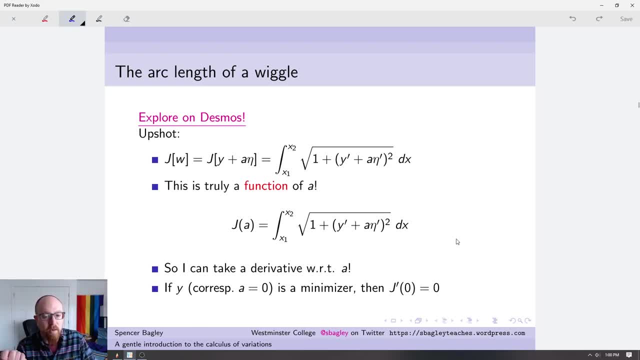 if my original function is a minimizer, that's the one that corresponds to a equals 0, which means 0 ought to be 0. And so I feel like that's a technical handle that I can use to calculate anything in this weird situation. Okay, Well, that's going to involve differentiating an integral. 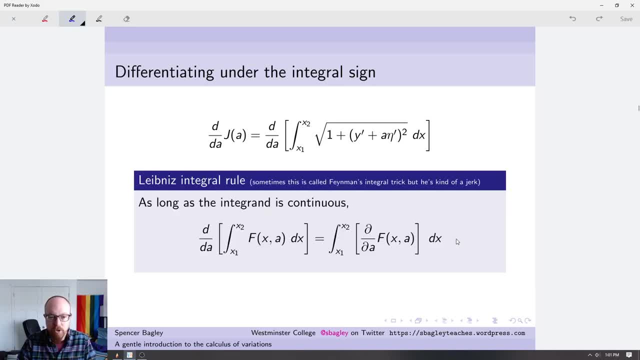 for which we're going to need to use a fun trick called differentiating under the integral sign or the Leibniz integral rule. Sometimes it's called the Feynman integral trick, but honestly he's kind of a jerk And so I don't want to stick his name on it, As long as the integrand is continuous. 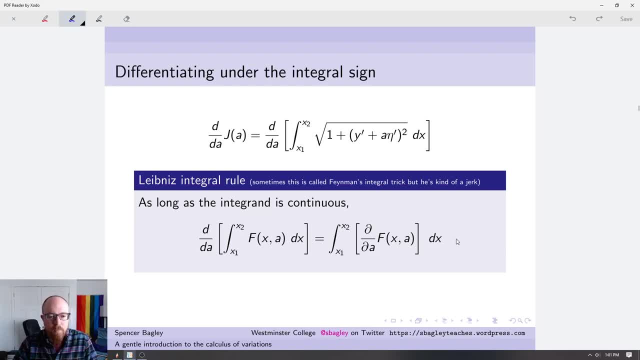 in the region that we care about, which I promise it is. you can interchange the order of the integral sign and the derivative sign, But then we need to think of the derivative sign as a partial derivative, because now there's one more variable going on. If this reminds you of Fubini's theorem, 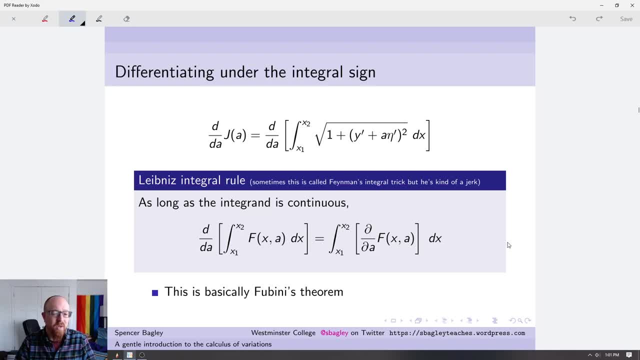 that's because it is basically Fubini's theorem. If this reminds you of Clairol's theorem, it's basically Clairol's theorem. I'm not going to prove it. You can think about what a proof would look like. It's not too bad. Speaker 1. 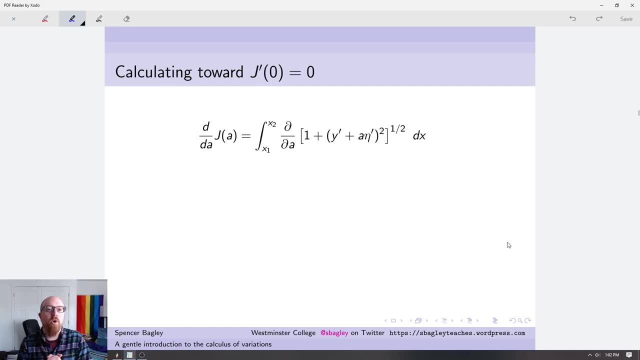 All right, So let's do this calculation. And I'm calculating toward the idea that j prime of zero ought to be zero. All right, So I've got the derivative of my function of a. I've done my differentiation under the integral sign trick. Let's do the calculation here. 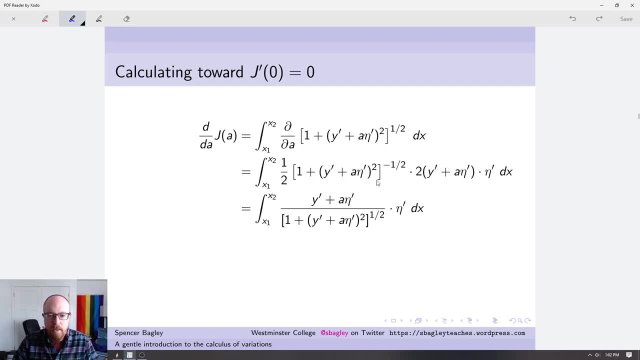 Works out to be this, And if I simplify a little, here's what I get. And now I want to think of this: when a equals zero right, And so I'm thinking of evaluating the derivative at the point a equals zero, and I'm told that I'm supposed to get zero right. 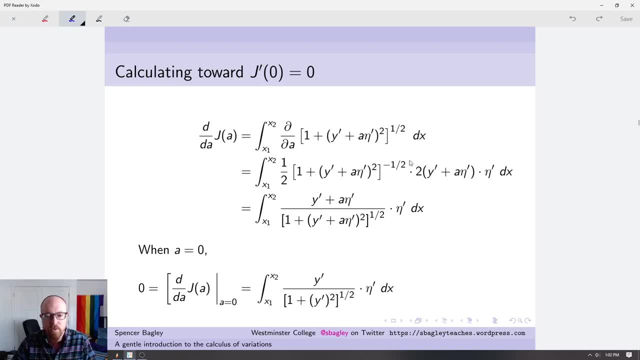 by my hypotheses, And here's what I really get when I substitute zero in: All these a's die and they take those eta primes with them that are inside, And the only eta prime that's left is this one that lives out here. Speaker 1. 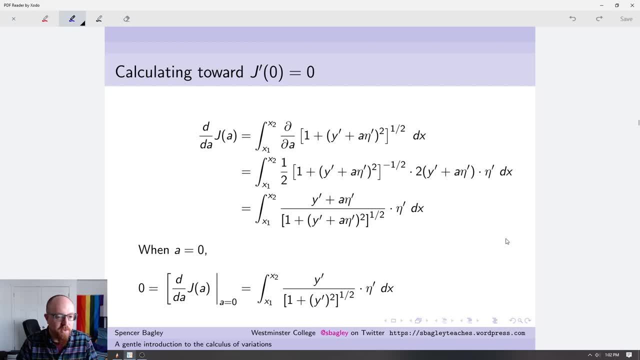 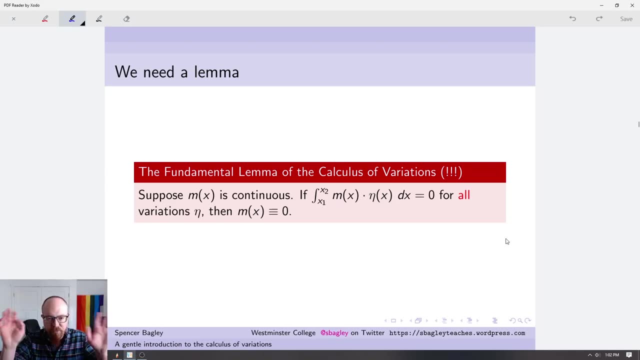 Okay, cool Boy. this is still a just a mess, though I don't really know what to do with this. What we're going to do with this is we're going to need a lemma, And it's called the fundamental. 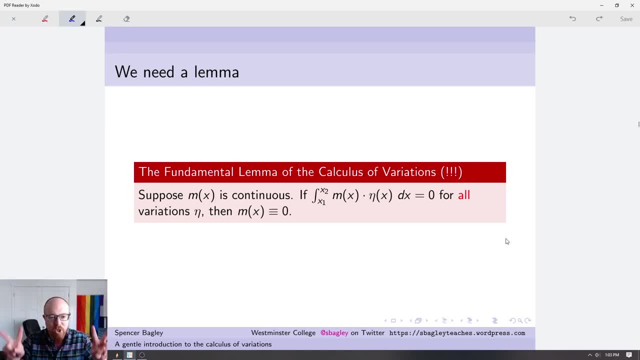 of the calculus of variations, and I love whenever something that's called fundamental comes up. here's what it says: if you integrate a continuous function against a variation and you get zero, no matter which variation you choose, well then the function has to be identically zero. right, the constant function zero. 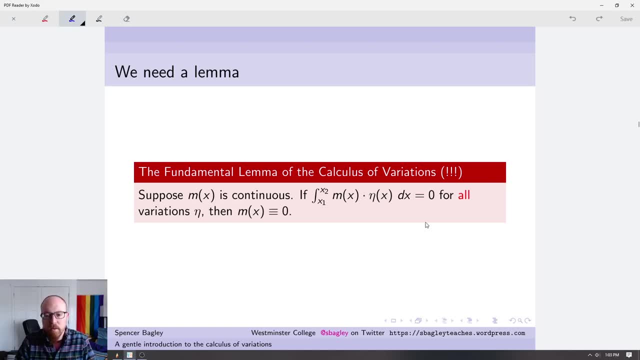 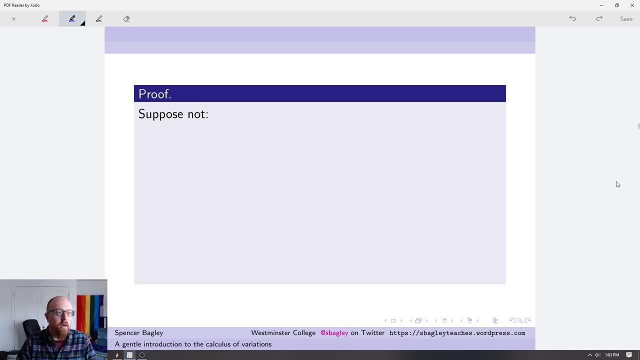 okay, let's see how the proof is going to go. the proof is fun. it relies on a little bit of analysis, but nothing too scary. we're going to do it by contradiction. we're going to suppose not. we're going to suppose that M is not the constant function zero, which means that somewhere it's got to either be. 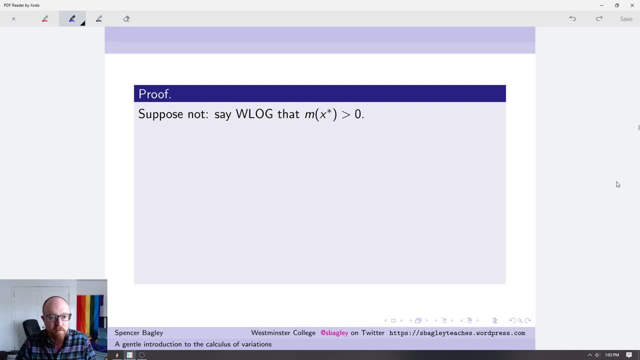 above zero or below zero, without loss of generality, we'll say above, there has to be some special x star where it's above zero. okay, and then our, our hypothesis was that the function was continuous, which means that I can take that point where we're above zero and I can fatten it up into a whole little interval where 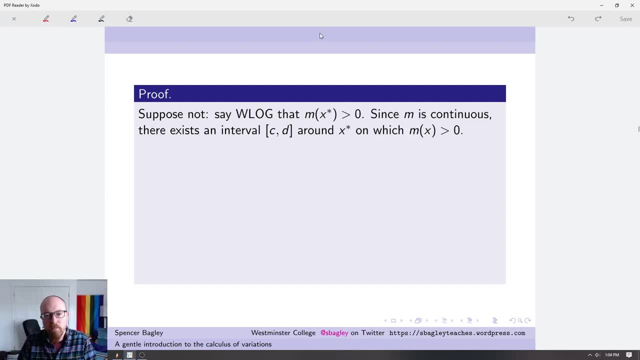 M is greater than zero. I think maybe a picture would be helpful here. here's my like x-axis right zoom. beautiful, that was nice and straight. here's my function M. if it's nonzero somewhere at this x star, well then it has. since it's continuous, it has to be nonzero on a little interval around. alright, cool so. 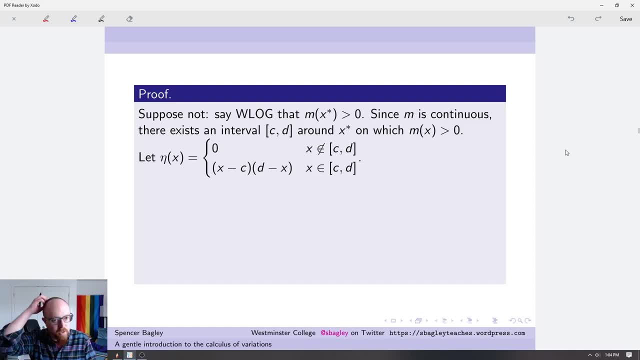 we're gonna say we're gonna make up a function, eta, which is zero outside of that interval, and then it does this little parabola thing on the interval. So I'll sketch that function Looks like this: Here is c, here is d, We're. 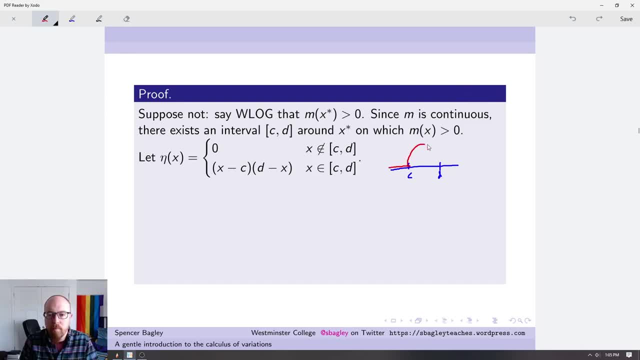 going to go zero, parabola zero. So this is clearly a variation, right, It satisfies our definition. It's piecewise c2.. It's zero at the endpoints because it's zero off of this small interval. All right, So by our hypothesis we were integrating m against this variation. We 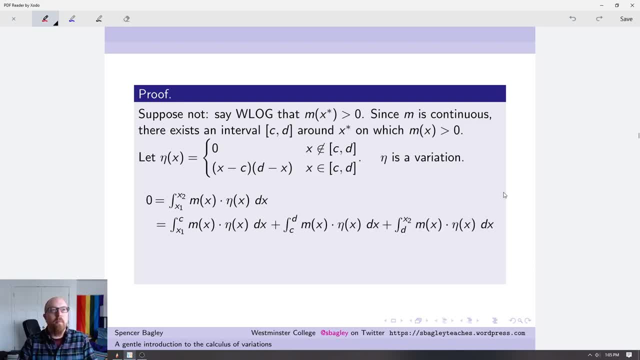 were getting zero. Okay, I'm going to split up this integral into three pieces, and I bet you can guess what those pieces are. You're right, They're precisely the piece between where we start in c, the piece between c and d, and then the piece between d and c. 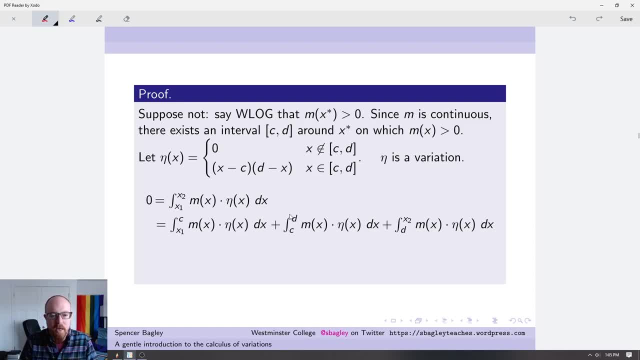 All right, And the reason that I'm doing that is because eta of x is in fact zero on this interval and on this interval, and so these two integrals will die. And then, what's more, this one right eta of x is positive because it's the upward parabola, by our choice, and m of x is 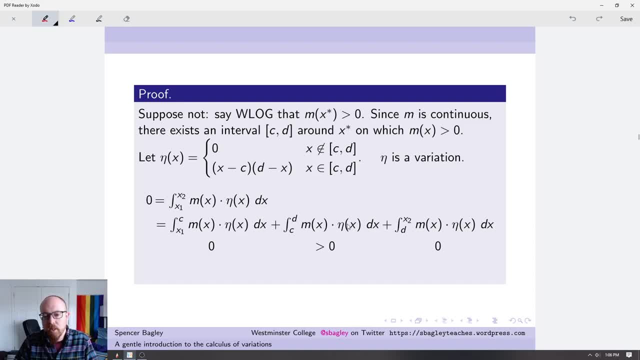 also positive on that interval. so I've got a positive things times a positive thing. If I integrate this word, I get the positive thing and I get the negative thing. So I've got a positive that I'm going to get something positive. There's my contradiction. Zero is greater than zero. 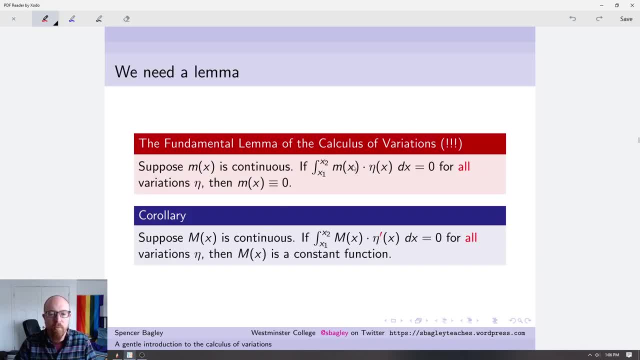 Okay, cool. So we have proved the fundamental lemma: If we integrate against a variation and we get zero, no matter which variation we choose, then our function is identically zero. Okay, here's a corollary. You may have noticed that we didn't have an eta in our previous thing. 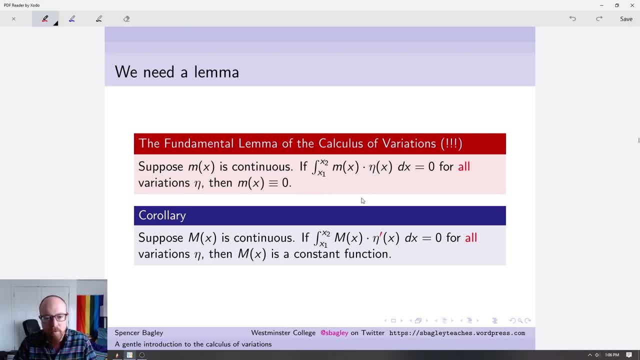 We actually have an eta prime. So let's see how that changes what we have. If I have a big M that's continuous and I'm integrating big M against an eta prime for any variation eta, well then M of x, big M is going to be a constant function. Okay, I bet you can guess how this is. 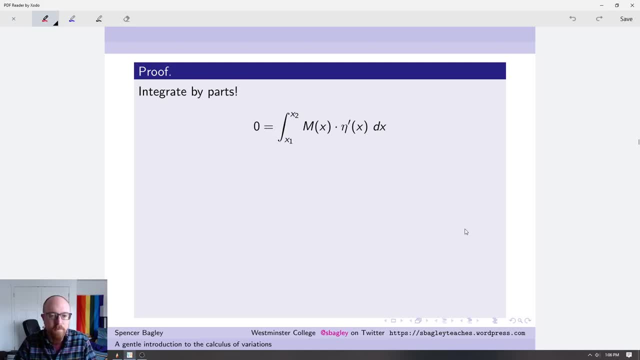 going to go. Here's how it's going to go. We're going to integrate by parts. I got to choose a u that I can take the derivative of and I got to choose a dv that I know how to integrate. Probably what I'm going to choose for dv is eta prime dx, so that v is eta of x. That leaves my u. 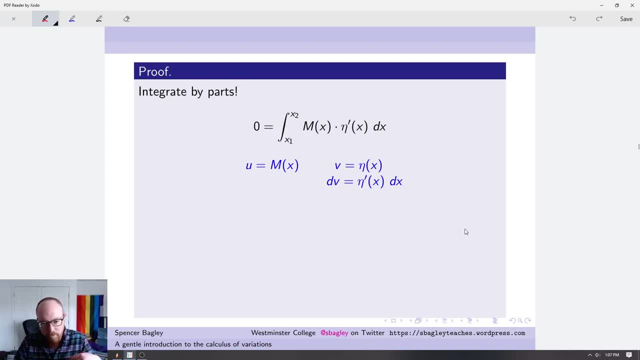 to be big M. My du would then be big M prime, which I'm just going to write as little m for reasons. Okay. and then if I throw this into my integration by parts formula, here's what I get. Here's my u, here's my v. and then the integral of vdu. Eta is zero at the endpoints, and so this: 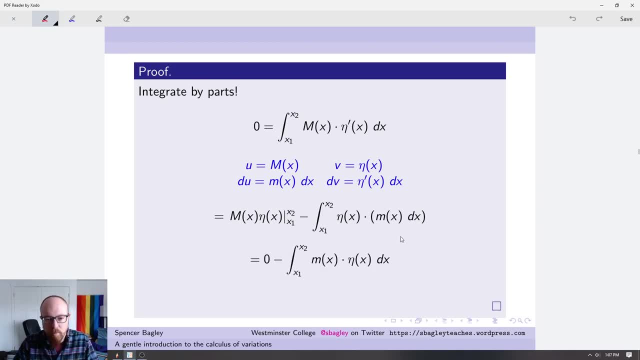 piece dies, which is nice, And so I just end up with negative this integral. But look at this: This is the integral that we just were in the situation of with the fundamental lemma. We can conclude, therefore, that little m is zero and little m was the derivative of big M. 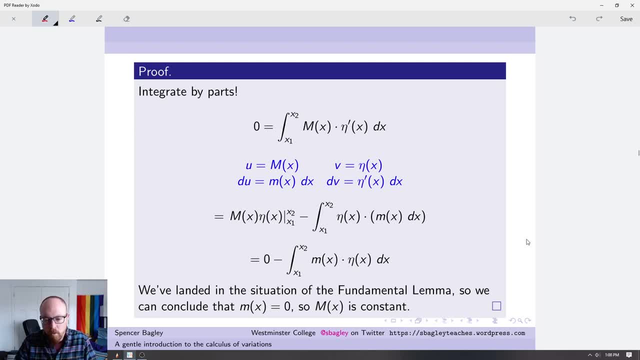 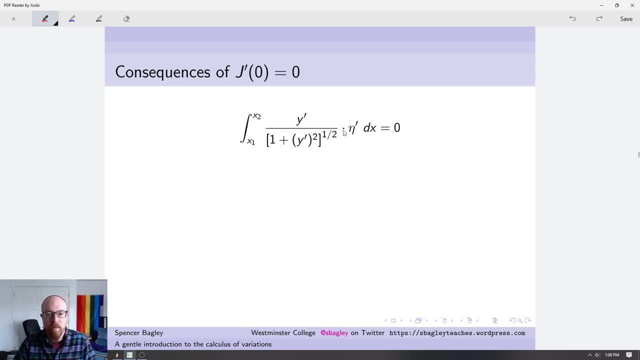 And so big M has to be constant. Okay, neat. What are we going to do with that? Well, here's what we have. We have some thing that is multiplied by the derivative of some variation, and we're integrating that and we're getting zero. That was the consequence of 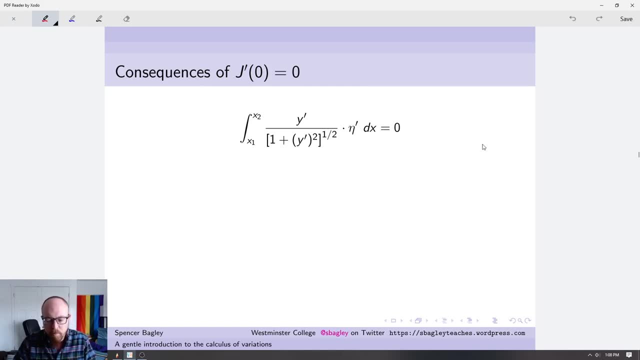 of zero ought to be zero, And so that means by the fundamental lemma, the corollary of the fundamental lemma, I should say: this thing that's integrating against at a prime ought to be some constant, All right, well, let's do a little bit of algebra. Here is what happens And what we end. 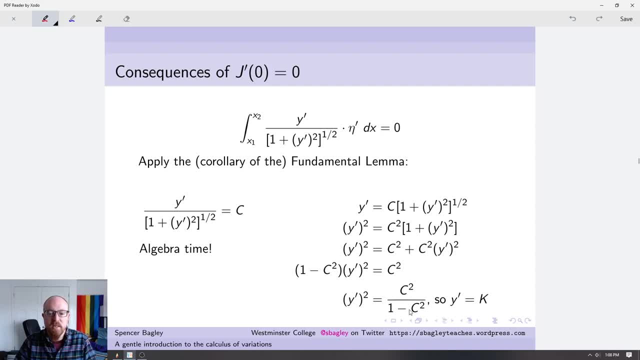 up with is that y prime is some constant like c squared over one minus c squared. but I don't really care, because c was arbitrary. Let's just rename that some new constant k. If y prime is a constant k, well then y is for sure a straight line. Hooray, we have proved what we thought was. 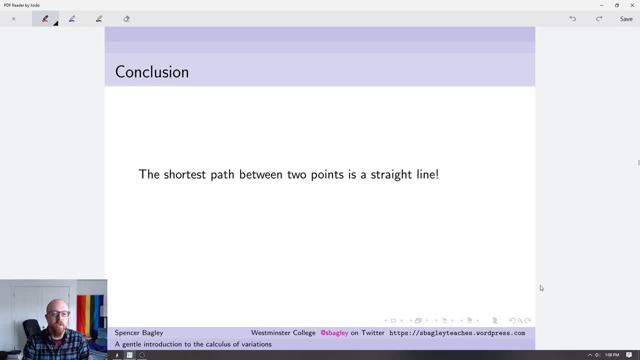 true. So here is what we have proved. We have proved that the shortest path between two points is a straight line. That's not actually what we proved. Here is what we really proved. If there is a shortest path between two points, it has to be a straight line. I am not going to get into the 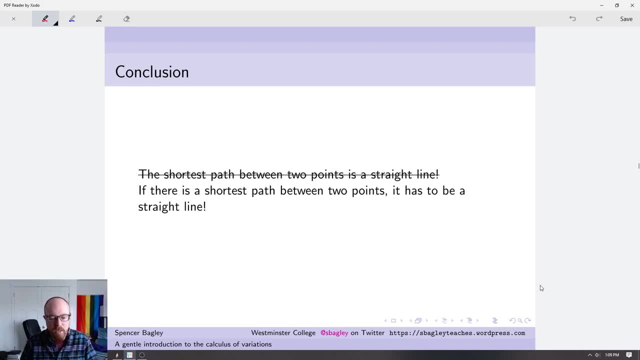 subtleties here of this sort of necessary versus sufficient distinction, because there's a lot more complicated math that you have to do. If you're going to deal with that, I think we're going to content ourselves with knowing something about the solution, if it exists, for the purposes of this 45-minute talk, All right. So let's sort of. 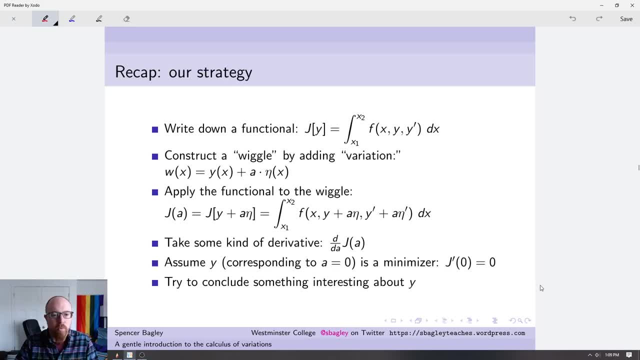 summarize the strategy that we engaged in here. We wrote down a functional in some way, We constructed a wiggle by adding a certain amount of variation, We fed that wiggle into the functional and here's what we got, And that was truly something that we were going to do. So we're going to 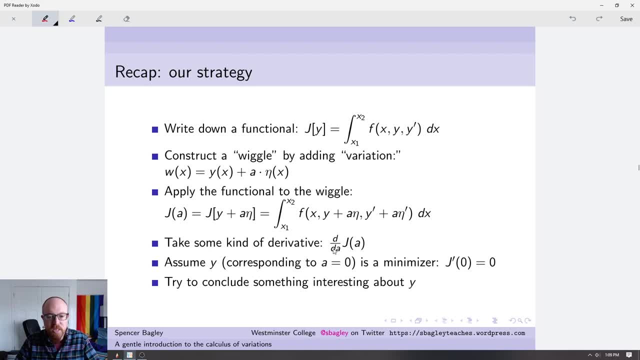 take the function of a, a single variable, And so we can do single variable calculus with it. We can take the derivative with respect to a. We're going to assume that we have a minimizer on our hands. Come up with j. prime of zero equals zero Calculate. And then, concluded, something interesting about y. 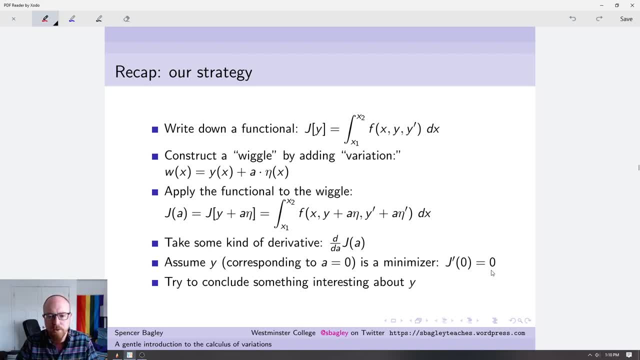 In our case that y prime was a constant. Let's see if we can apply this strategy. now that we've done, now that we've thought our way through this whole wiggle and variation thing And gotten to the fundamental lemma, I bet that we can apply this strategy more broadly pretty quick. 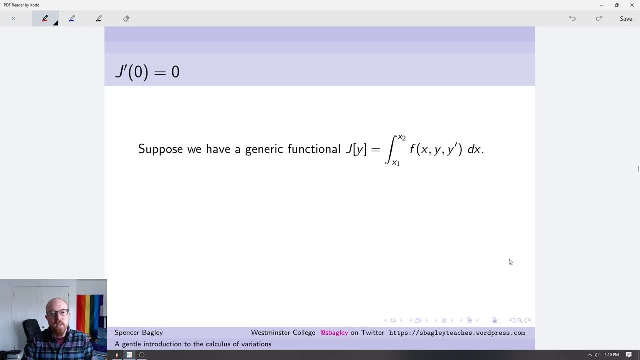 So let's think about how we could do that. Let's say that we just have some generic functional with some generic integrand here. If we do our whole, you know, apply to a wiggle and take the derivative thing, here is what we're going to get. if we write down that j prime of zero equals zero, Well, the 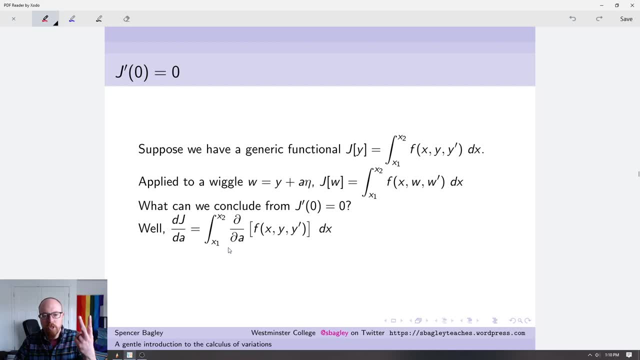 derivative of j is the integral of the partial derivative right Differentiating under the sign. What is that partial derivative going to look like? It's going to be weird. So f really depends on x and it depends on w and it depends on w prime, And x doesn't depend on a, but both. 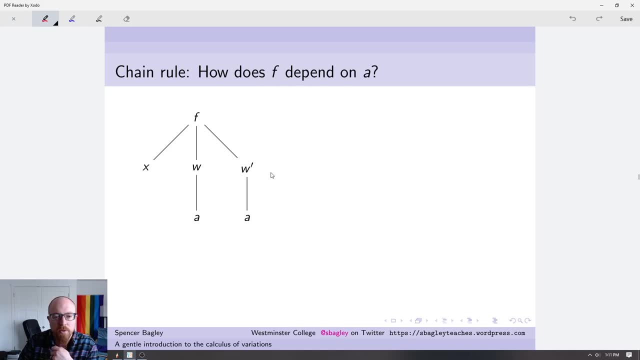 w and w prime depend on a, And so then, if we use the chain rule, we can write down an expression for partial f, partial a, which is this business, All right, And then. well, okay, So since w was y plus a times eta, that means that the partial of w with respect to a. 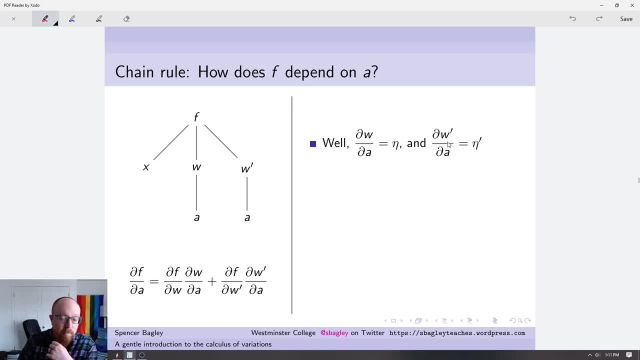 is going to be eta, And similarly, the partial of w prime is going to be eta prime. So we can throw those into this here and here's what we get. And then we were really interested when a equals zero, And when a equals zero, w is just y right If we collapse out, the amount of variation. 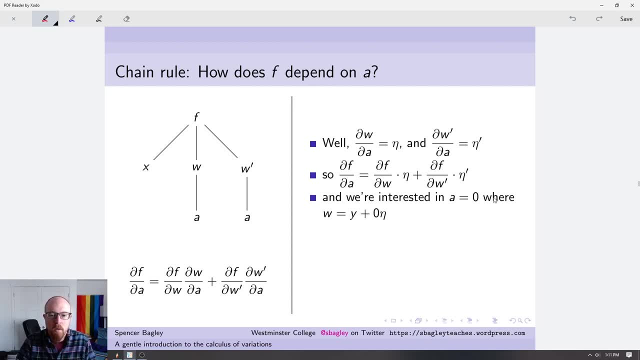 we get our original curve. That was sort of the point, Sure. So then, as far as we ever cared, partial f partial a is going to be partial f partial y times eta. partial f partial y prime times eta prime. Okay, We're going to do. 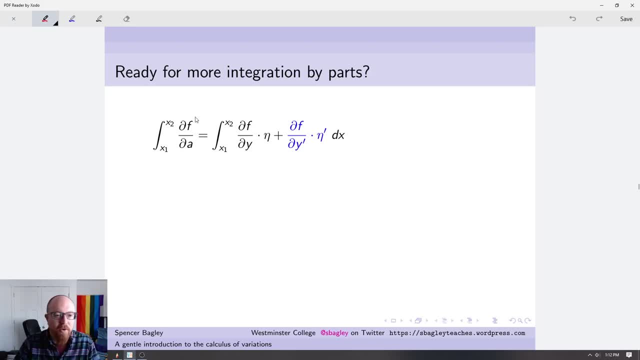 some more integration by parts. Here we go. We are. oh, I forgot a dx here. Pretend it's there. We were integrating the partial of f with respect to a. We can substitute in this. we're going to do some more integration by parts here, because any time I see something multiplied. 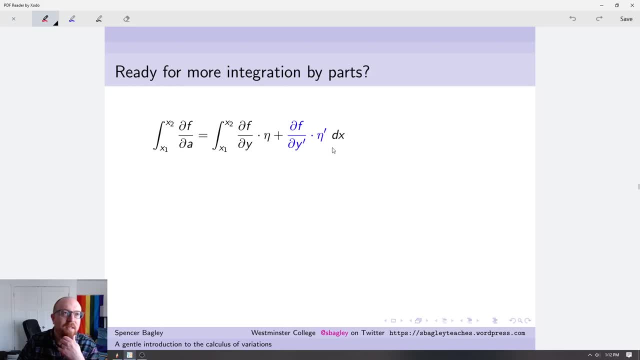 by a derivative and I'm integrating it. I like to use integration by parts to get rid of that derivative. That often results in something nice happening. I think again, the clear choice for dv is our eta prime, which means that v is going to be eta, And then that leaves a partial f, partial y. 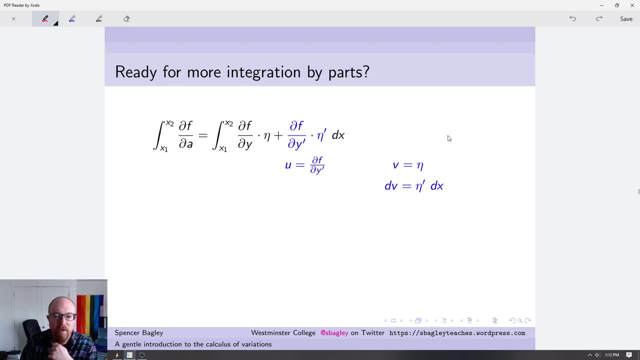 prime to be our u. We are going to take the derivative of that with respect to x, which is weird, But that is what we got to do here, because we are integrating with respect to x. All right, So then the second term: let's integrate by parts and put all the 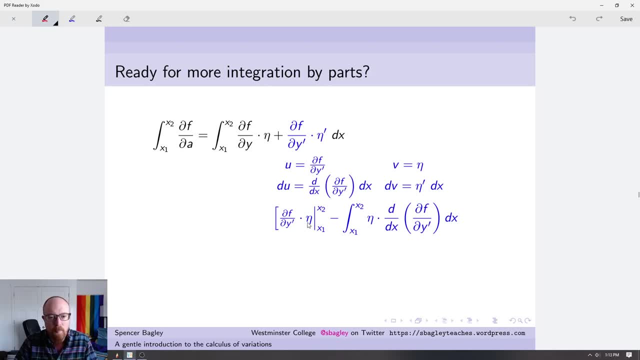 pieces together. Here is our uv. Again. since we're evaluating from x1 to x2, and eta is a variation, this will die, It'll go to zero. And then we've got the integral of v? dv, which is the. 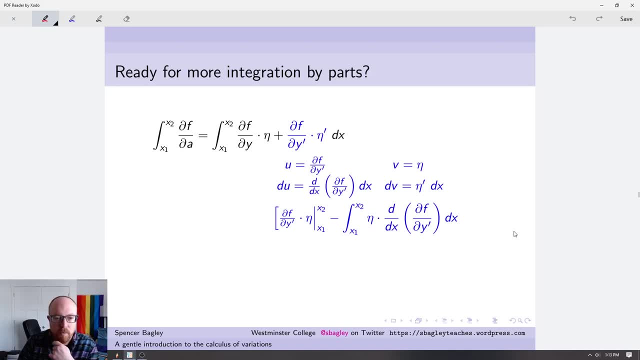 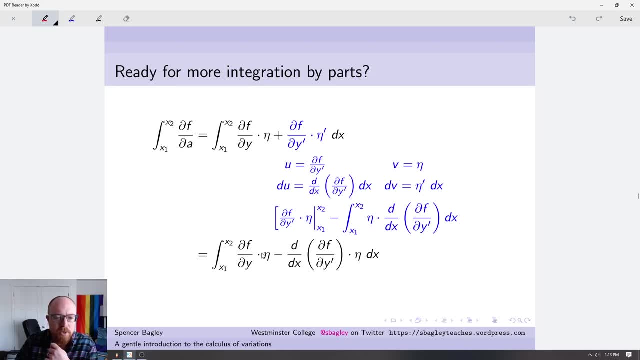 whole big integral. And here is what I get. Notice that I can factor out an eta now And that leaves me behind this red part. So I've got this red part and it was multiplied by eta. Oh, but this was integrating to zero, which means that once more we have landed in the situation of the. 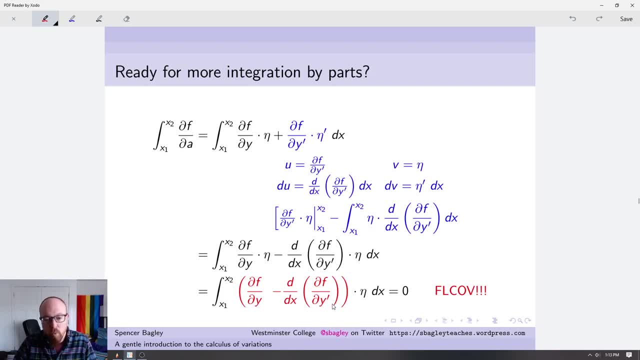 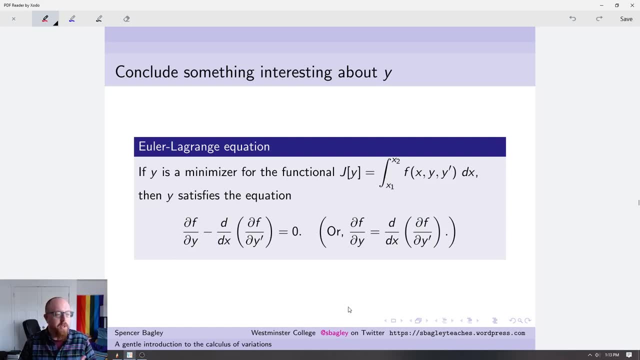 fundamental lemma that we proved Cool. This means that this quantity has to be identically zero. This is called the Euler-Lagrange equation. This is what we can conclude. that's interesting about why it has to satisfy this partial differential equation. I'm going to write it. 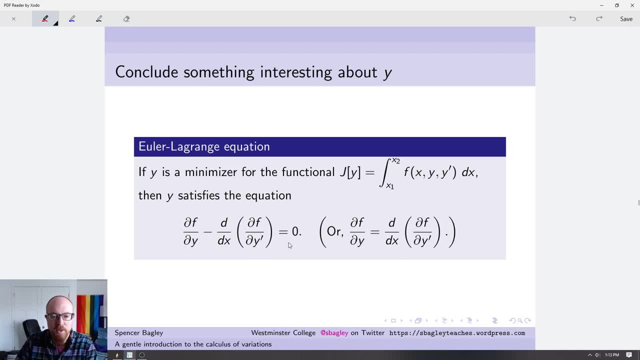 in two ways: Either that quantity that was multiplied by eta has to be zero, or if you just add this over, you can see the partial of f with respect to y has got to equal the x derivative of the partial of f with respect to y prime. Hold that thought, because we're going to see it again. 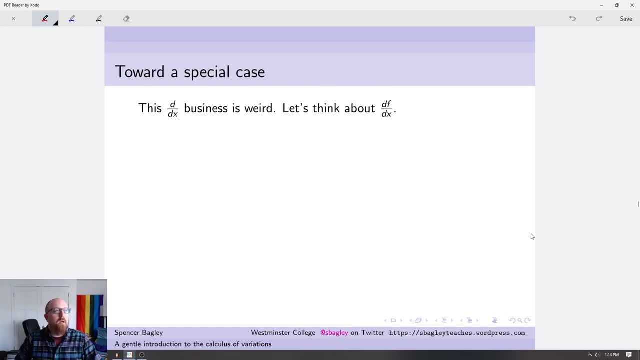 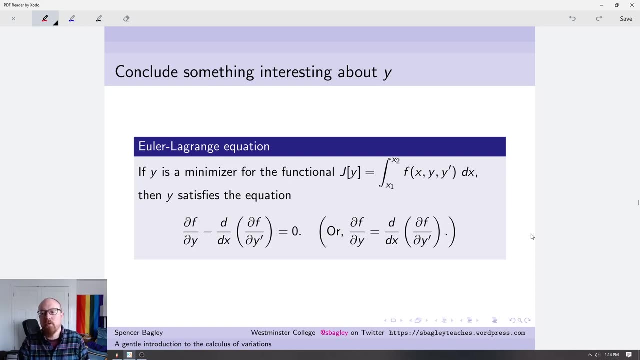 on the next slide. Okay, I want to think of a special case of this, because in general this partial differential equation is kind of hard to solve and it's a little more powerful than we really need. So here's a special case. Look, I've got the derivative, with respect to x of some other thing. 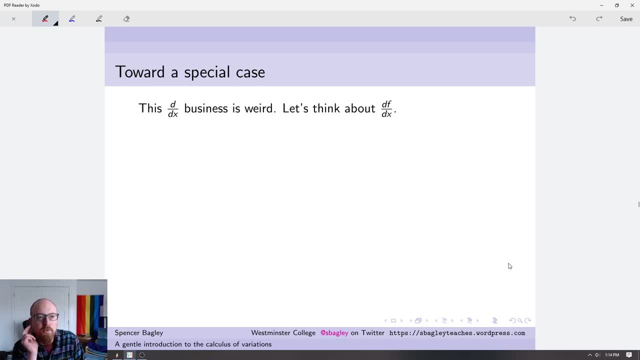 and that feels weird to me. I think it might be useful for us to go back to our original integrand and think of its total derivative with respect to x. And so here again is this tree diagram. Looks very similar to the one we drew before, but this time we're looking at the 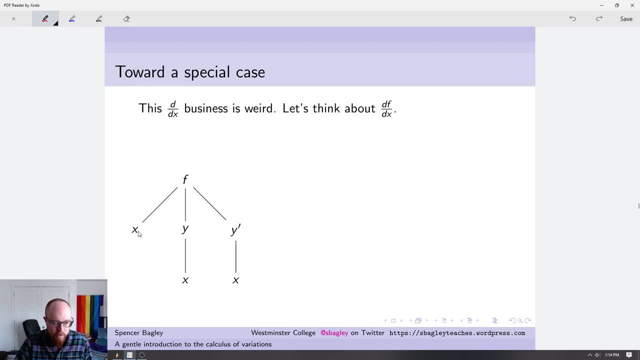 dependencies on x instead of on a. So f depends directly on x and it also depends indirectly on x through its dependence on y and on y prime. And so if we hit this diagram with the chain rule, we get the following: So the total derivative of f with respect to x is the partial of f with 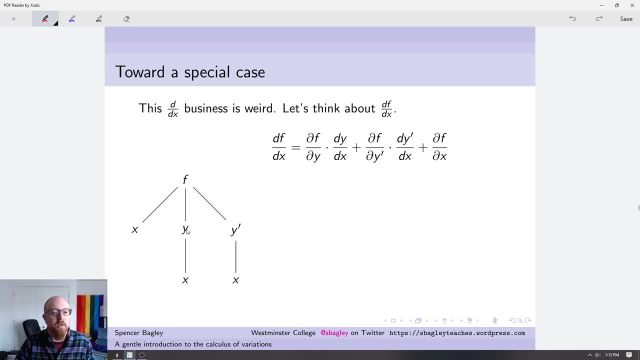 respect to y times, the partial- excuse me, the derivative- of y with respect to x. That's not partial because y doesn't depend on anything else. And then we got the partial of f with respect to y prime, and then the derivative of y prime with. 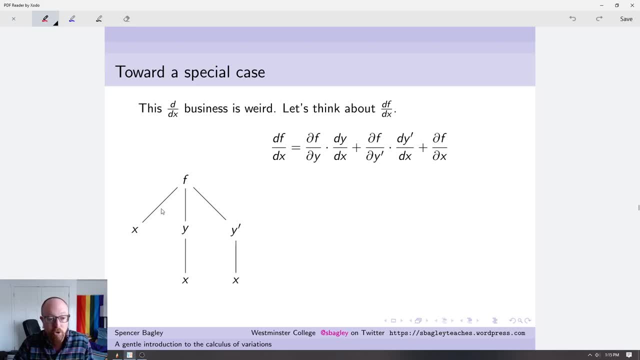 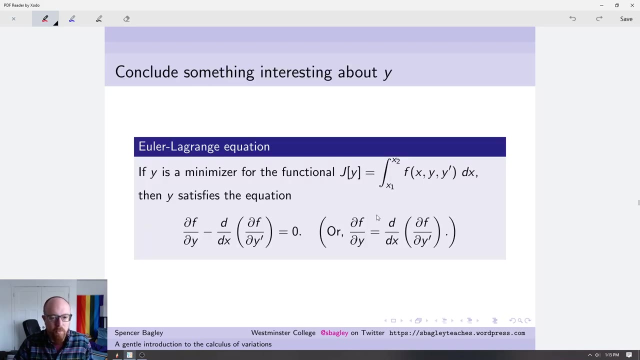 respect to x. And then we got the partial of f with respect to x. that reflects f's direct dependence on x, maybe. So the thing that we just learned from the Euler-Lagrange equation was that the partial of f with respect to y is actually just the x derivative. 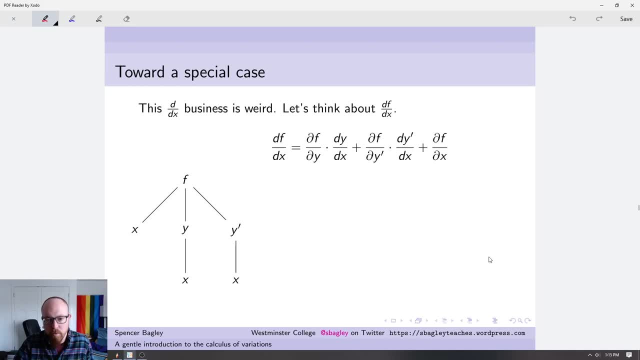 of the partial of f with respect to y prime. So we can replace this here with that: dy dx is y prime, dy prime dx. I'm going to call the derivative of y prime. Look what I got here. now I've got the derivative of a thing times something else. 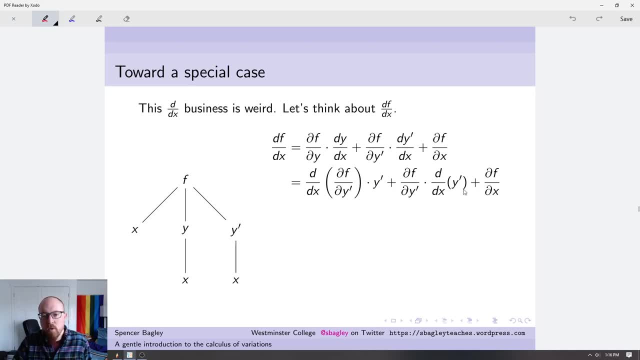 and then I got the thing times the derivative of the something else, which sounds to me a heck of a rule, except I'm going to apply it backwards. And so here is what I get: That is just the x derivative right of this thing times this thing. So that's cool, And then I just have 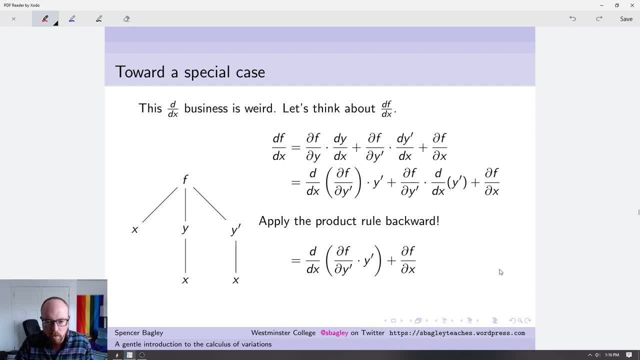 this partial depth with respect to x trailing out here. All right. So then, if I just subtract this term over, I end up with this equation, which I think you can see is true. So I said earlier that a lot of functionals that we care about are not going to depend explicitly. 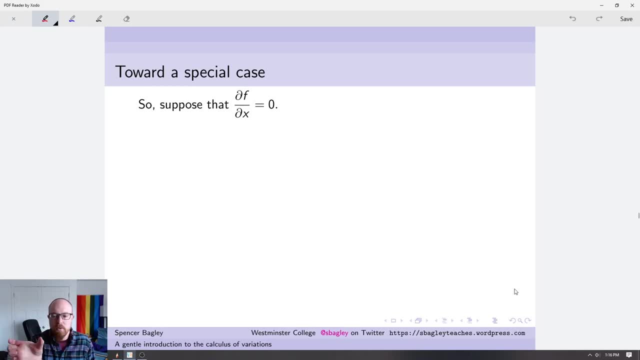 on x because things are autonomous and don't shift, don't change when you shift from left to right, Right. So as long as the integrand of the functional doesn't depend on x explicitly, I bet that we're going to get a nice special case because this: 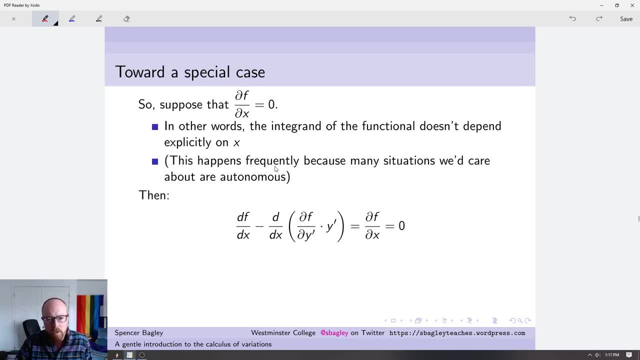 partial of f with respect to x is zero. So here's what we've got, And we can think about just adding this back over now and then integrating both sides, or you know, factoring out the derivative quote unquote and getting this, and then integrating both sides, And so we 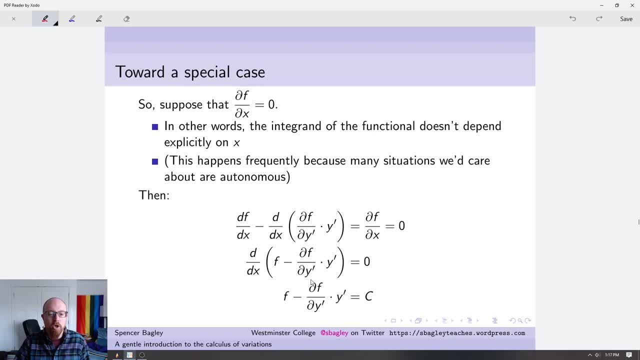 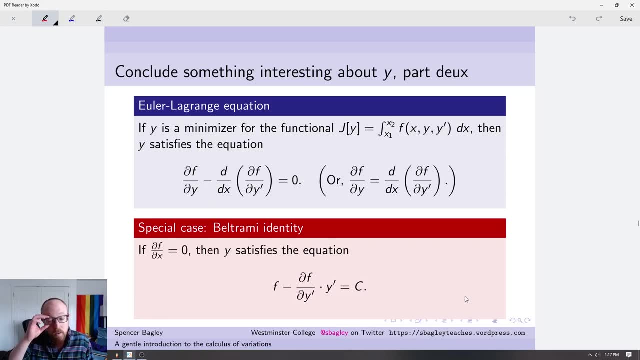 could conclude that f minus the partial of f with respect to y prime times, y prime should equal some constant, And this is called the Beltrami identity. So this is a special case of the Euler-Lagrange equation, in the case where the integrand doesn't depend explicitly. 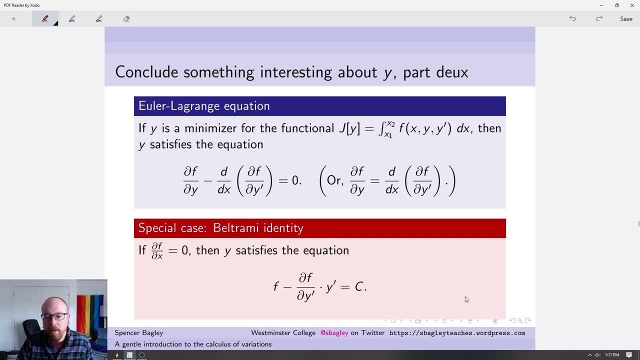 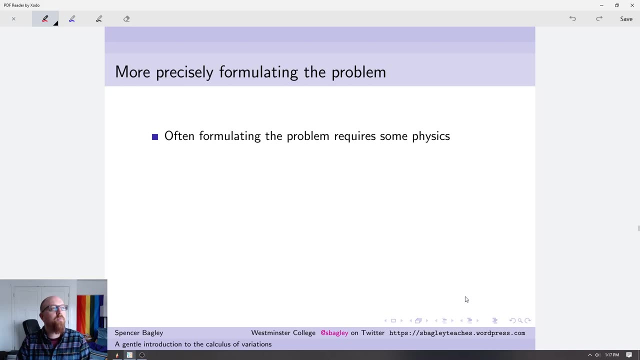 on x. Okay, fun. I feel like we now have some tools that we can confidently apply to various situations that we may find ourselves in. Let us return to the catenary. Sorry, that was a bad joke. We need to more precisely formulate the problem right. Originally, we 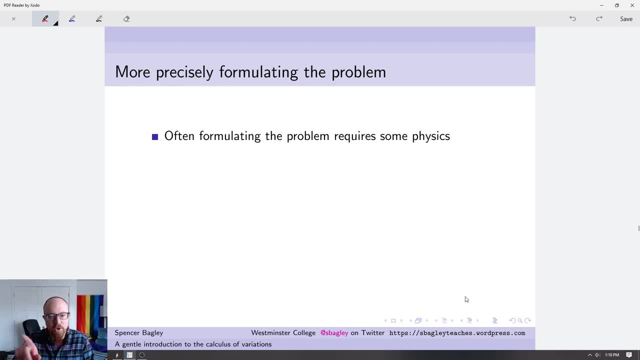 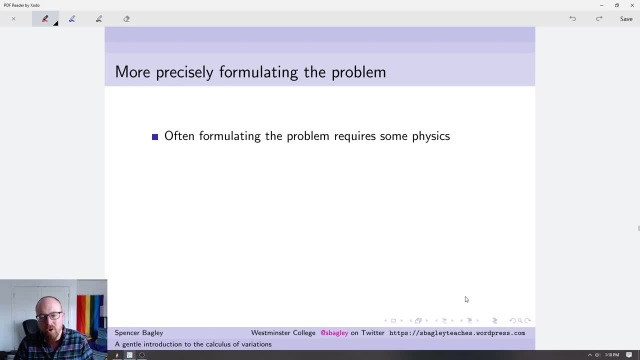 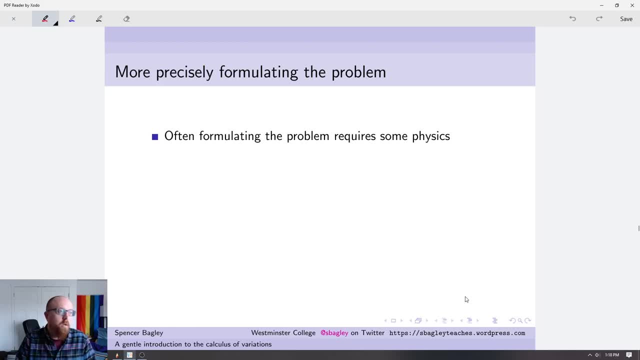 the problem more precisely, The operative thing here is that things generally in nature want to minimize their energy, And the particular kind of energy that we're interested in here is gravitational potential energy. If the chain is suspended from two points, it wants to hang in a way that minimizes the gravitational potential energy. There's also the length. 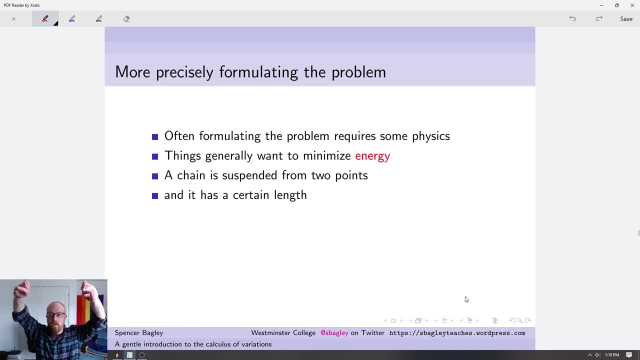 of the chain that we have to think about. right, If I have a longer chain, it's going to go like whoo, as opposed to a shorter chain. that's going to go like whoop, whoop, whoop. 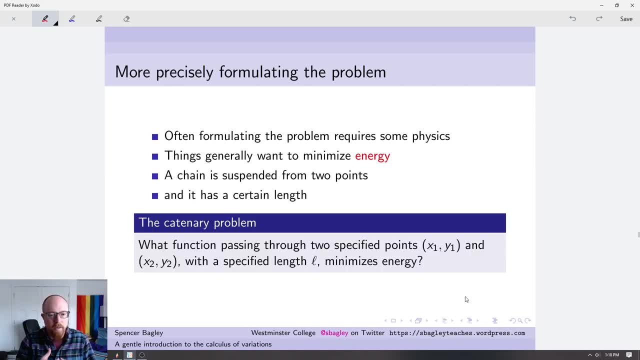 So here is a more precise formulation of the catenary problem. What function? passing through two specified points- x1, y1, and x2, y2, with a specified length, minimizes the energy, the gravitational potential energy. Okay, I'm going to need a functional. 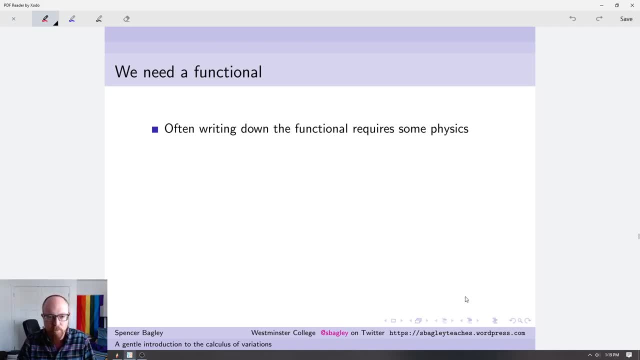 and again we're probably going to have to activate our physics brain for this. That's pretty common. Like I said, energy in this case is probably gravitational potential energy We are going to slice, approximate, integrate. again We're going to think of a little chunk of the chain as a point mass. 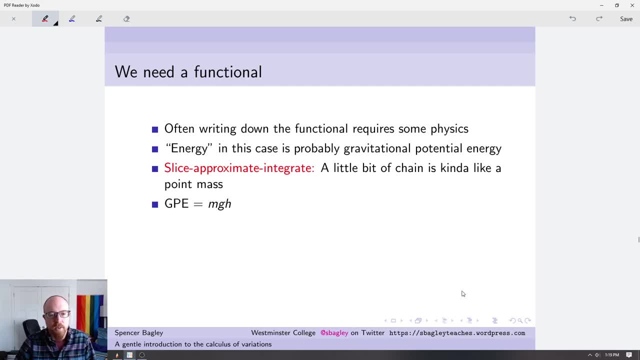 and then the gravitational potential energy of a point. mass is the mass of that thing times, uh, acceleration due to gravity, times the height that it has above the ground. Okay, Well, the, uh, the mass of that little thing is going to be like. 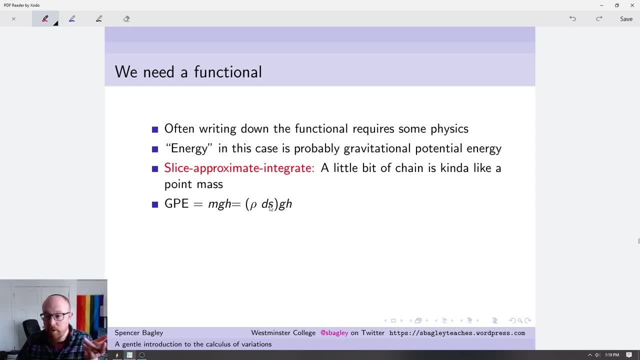 the mass density of the chain times ds- Oh look, there's that ds that I told you was going to show up again. Multiplied by g, multiplied by the height. I am going to assume here that the mass density of the chain is constant. 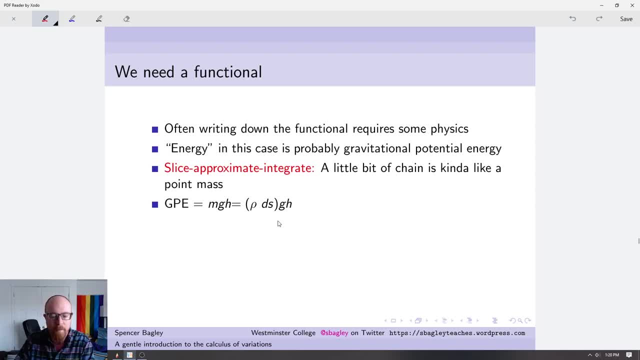 which is a pretty decent assumption, because otherwise things would get real bad. Um, okay, so I'm just going to rearrange some stuff. Okay, So I'm going to pull this out here. uh, pull my two constants out. um, 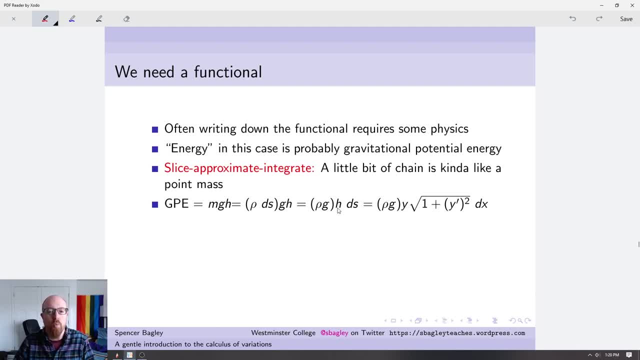 and then I'm thinking of of the height as y right y, of x, the function, and then ds: uh, was this that I told you to remember? Um, okay, neat, So then I just need to integrate that. 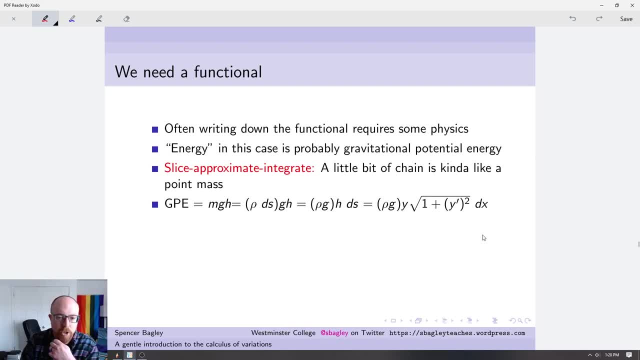 and I get the uh, the total gpe of the uh, of the whole chain. Um, and in particular, since we're minimizing, we're just going to like take the derivative of this thing and set it equal to zero. 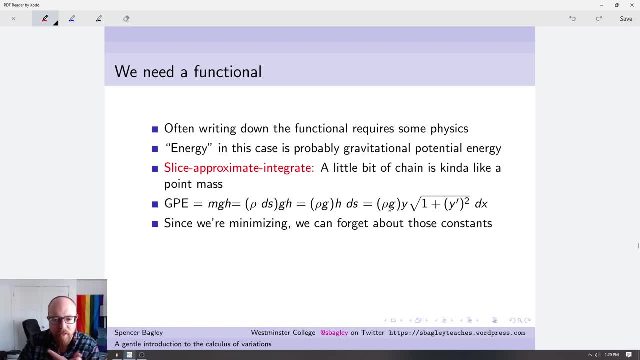 So these constants are just going to hang out, and then we can divide them over to the zero side, so we don't even need those. So here's our functional Um. we're now our integrand is y times the square root of 1 plus y prime squared. 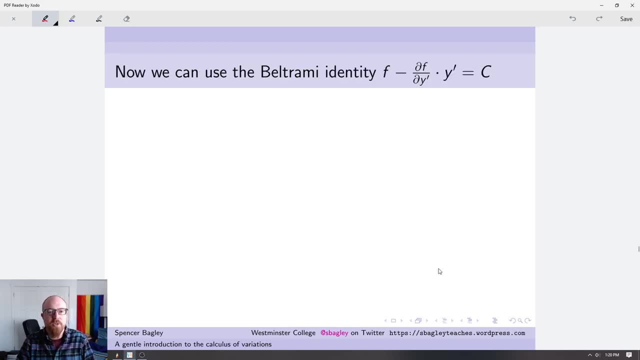 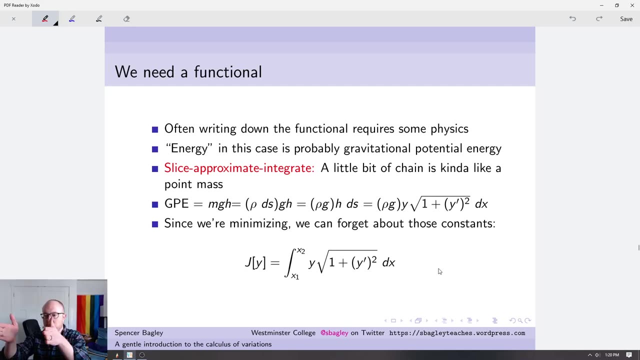 Okay, Um, well, that's neat. We can probably just immediate. I'm noticing that there's no x's in there, right? Um, this is an autonomous situation. If I shift the chain from from left to right, probably nothing is going to change. 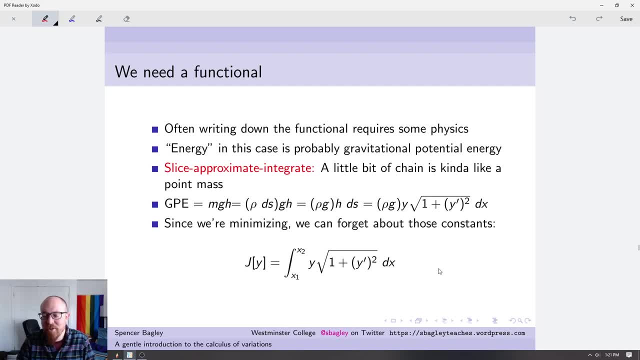 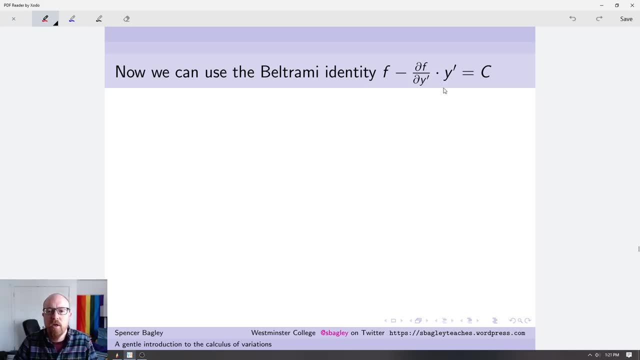 because gravity is the same If you move one foot to the right. um, that means that we can use the Beltrami identity, All right. So we're going to need to do some calculations, We're going to need to figure out y prime. 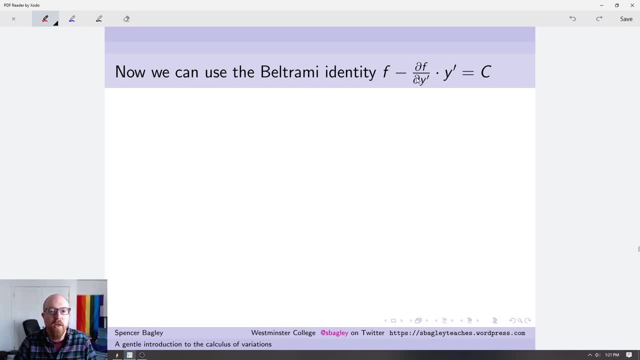 And uh, no, I'm sorry- We're going to need to figure out the partial of f with respect to y prime, And then we're just going to multiply that by literally this symbol: y prime, Um. here's our function. 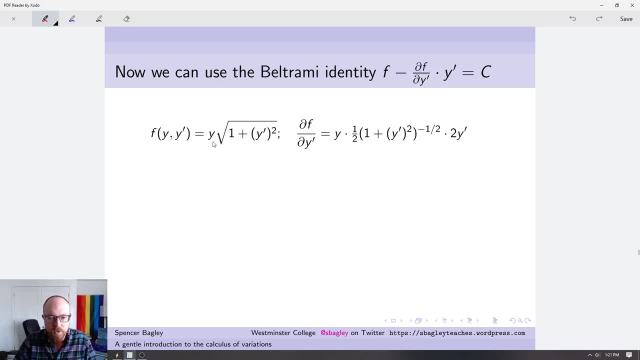 Here is its partial with respect to y prime. Notice, as far as y prime cares, y is a constant. I'm doing this very formally. Yes, there is a relationship there, but just symbolically speaking, y prime considered as a different symbol than y. 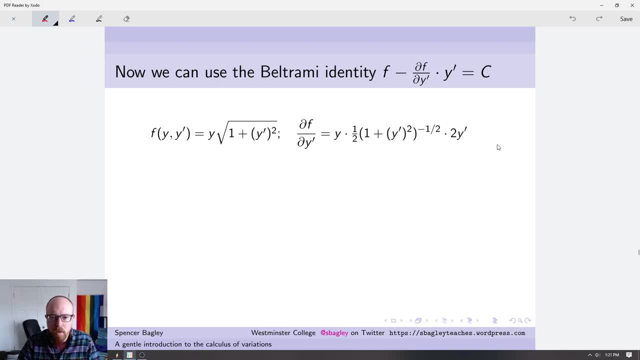 um is, is what we're taking, the derivative with respect to? uh, do a little algebra clean that up. It looks like this: Um so then, if I throw these pieces into the Beltrami identity, here is what I get. 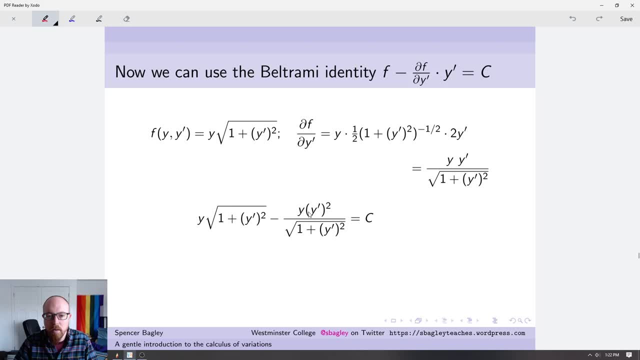 Here is my f, Here is my uh. partial f, partial y prime. Now that I've multiplied it by y prime, this y prime ends up being squared. Okay, And then the difference of those is supposed to be a constant Neat. 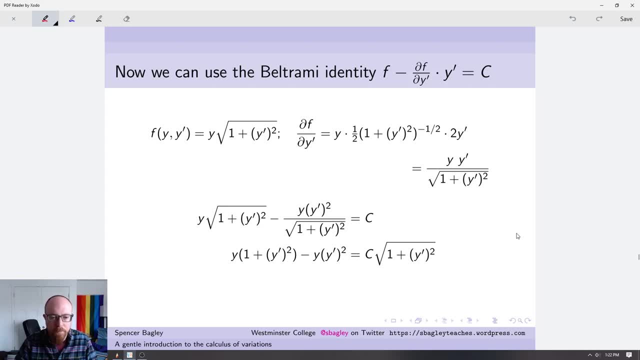 Um, I'm going to clear that denominator because the square roots are freaking me out. Um, I can now distribute this y through, and then some stuff is going to add to zero, And so here's what I get. That's pretty decent. 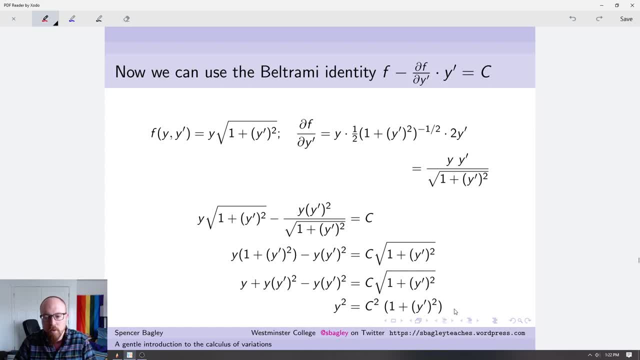 This doesn't look like too bad of a differential equation to solve, which is kind of surprising, Like this seemed like a way way harder problem than would just be amenable to attacking it with a simple differential equation. Um, this is even a separable differential equation. 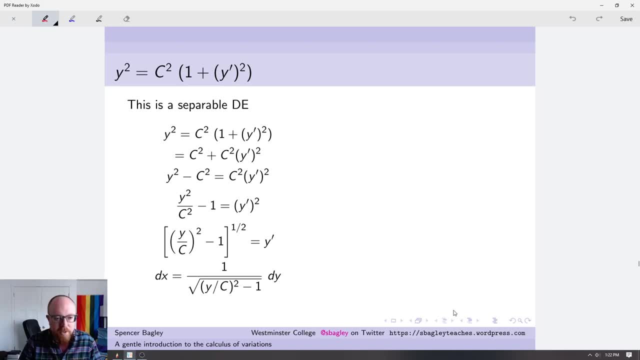 Um, here's the algebra for that. Um, I'm not going to talk through it cause that's boring. Um, you can integrate this. It's not nice And I I encourage you to try. There is a particular substitution that will make it nice. 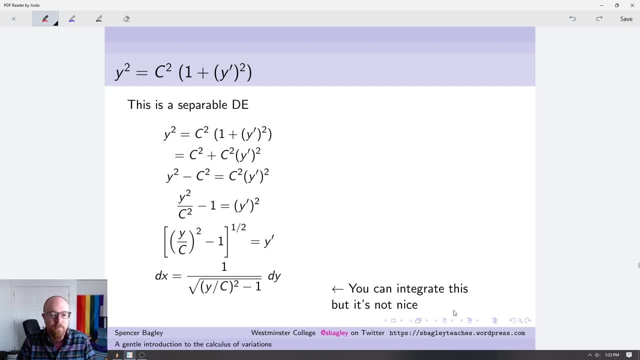 but um, I'm not going to say what it is for just a second. Um, I wonder if there's another way that we could approach this problem, though, Um, I like to. I like to say that differential equations is the study of dirty tricks. 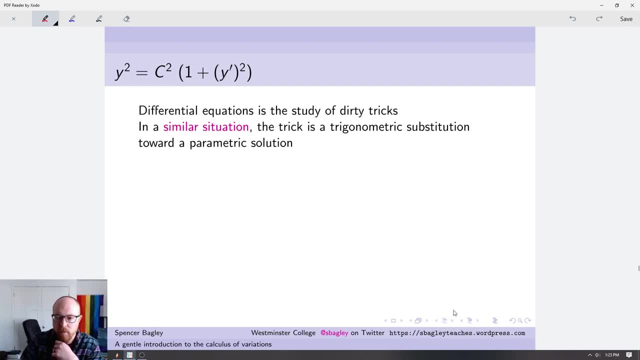 Um, there's a very similar situation- Click on that link if you want to read the details- where the correct trick is a trigonometric substitution. Uh, and then we're going to work toward a parametric solution instead of an explicit solution. 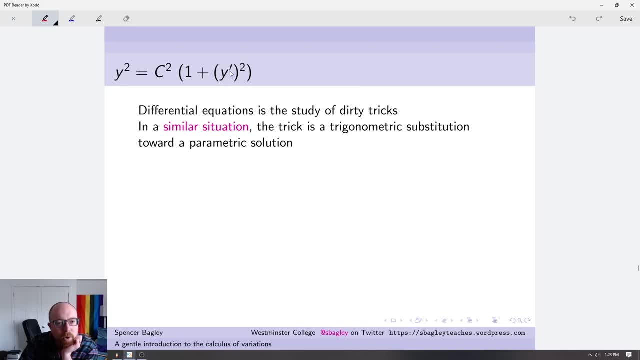 Um, you can see, if my y prime was, let's see, I guess, a tangent of theta, then I got one plus tangent squared, and that should be secant squared, and then maybe some good stuff happens. Um, so let's try that substitution here. 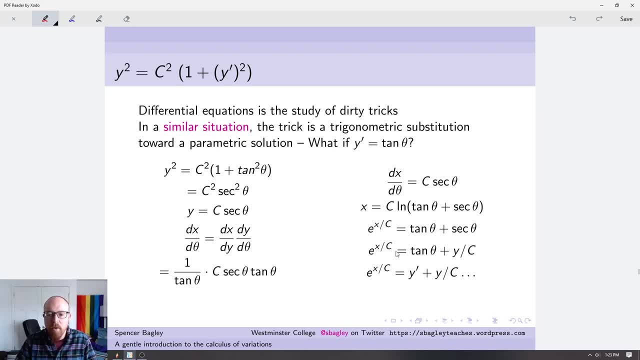 Um, I had spun my wheels with this for a little while. I think you end up getting something that works. Um, if you make this substitution and dink around with it, you end up with this, which is a- uh, first order. 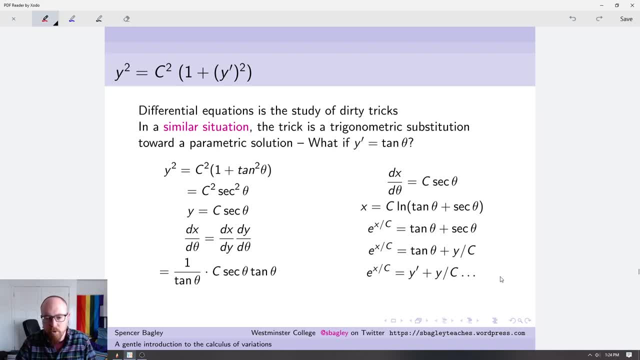 uh, non-homogeneous, uh differential equation, which is fairly straightforward to solve. This works, Um, I think it feels like the wrong trick. I think there's maybe a cooler, funner trick that we can do, And let's see what that trick is. 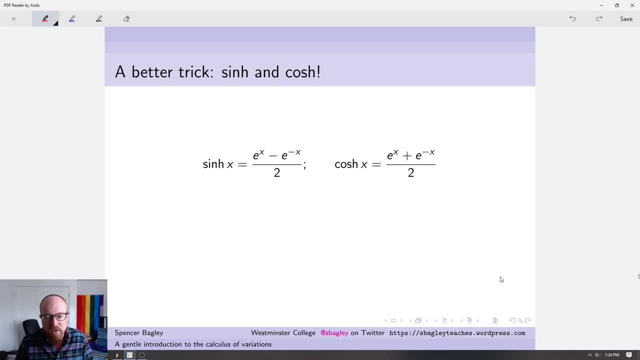 The trick is cinch and cosh. These are called the hyperbolic sine and hyperbolic cosine. Here are their definitions. They are related to our usual uh, circular sine and cosine, um in a particular way, Um. 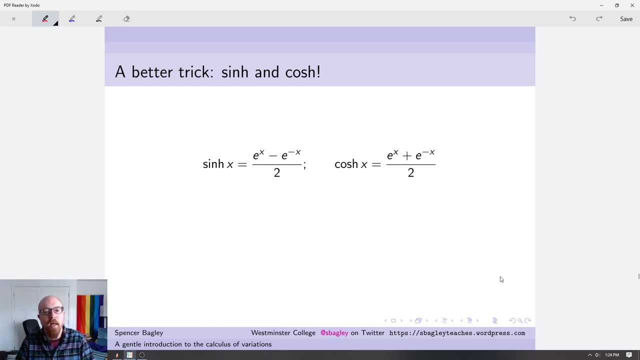 if you think hard about the real and imaginary parts of e to the i, x, uh, I think you can see what is going on. I'm not going to say too much about it. Um, here are the things that you care about. 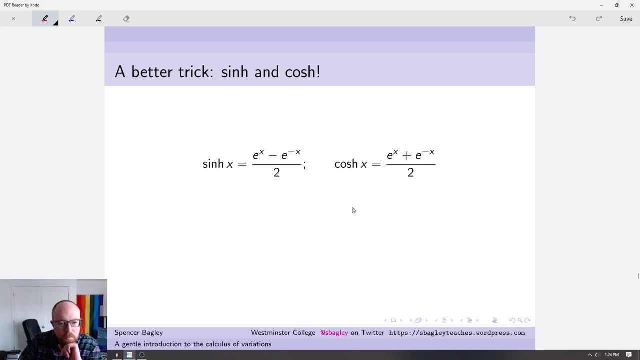 uh, from these definitions, And you can check that these are true. Um, if you take the derivative of cinch, you get cosh, And if you take the derivative of cosh, you get cinch, which is like one step nicer than the relationship between sine and cosines. 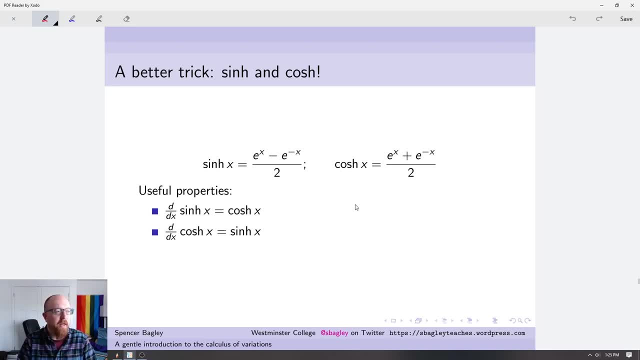 derivatives. Um, and there's also sort of a Pythagorean-ish identity going on here As well, which is this: uh, the square of cosh is equal to one plus the square of cinch, So this is close to the Pythagorean identity for sine and cosine. 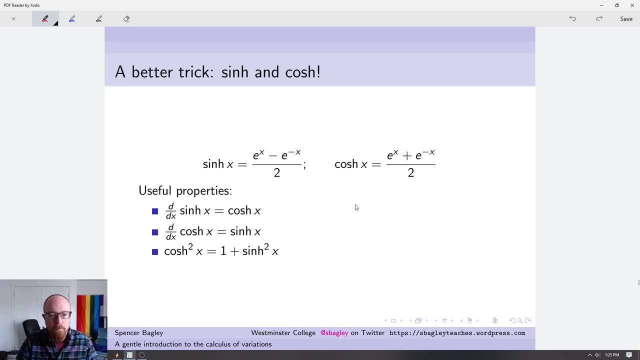 but sort of things are in different places. Um, and in particular, I'm liking that I have a one plus something squared. um, because that was what my differential equation looked like. Okay, so here we go, I've got my one plus something squared. 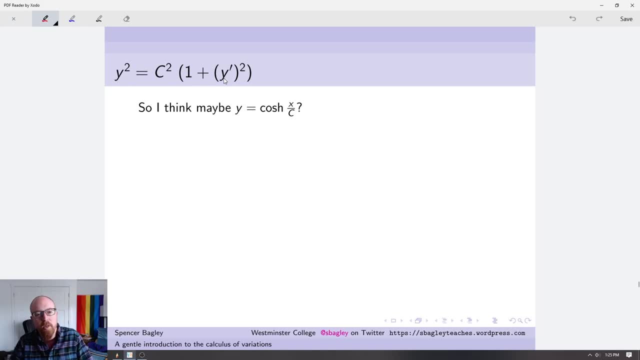 If I threw in like a, like a cosh, here, I probably win Um. no, I'm sorry, If I throw in a cinch here, I probably win Um. but there's also the c, and then let's see. 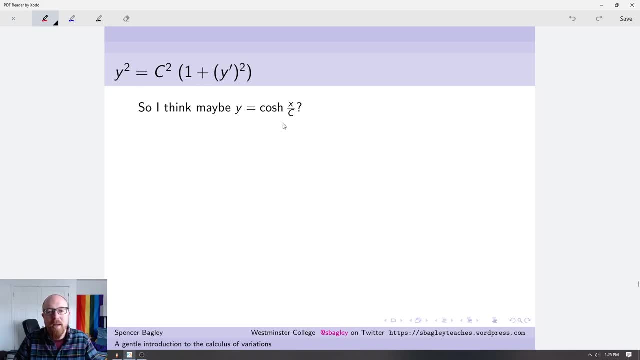 if this was a cinch then I think my y would have to be a cosh. I'm going to guess, um, that y is the cosh of x over c. Um, let's see if that works. Uh, y prime is going to be one over c times the cinch of x over c. 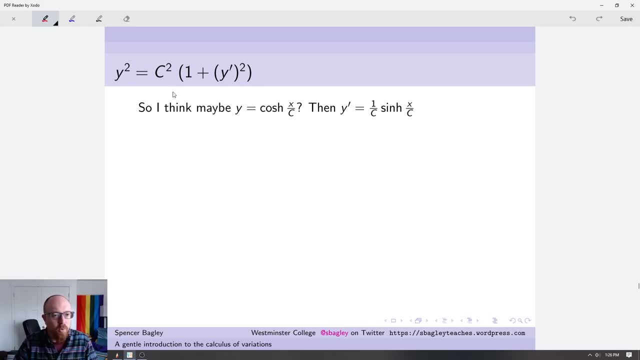 Which I'm hoping will sort of uh, cancel out that c squared that we have up here. Um, let's see if that works. Uh, one plus y prime squared is this business, which I don't think is going to add up correctly. 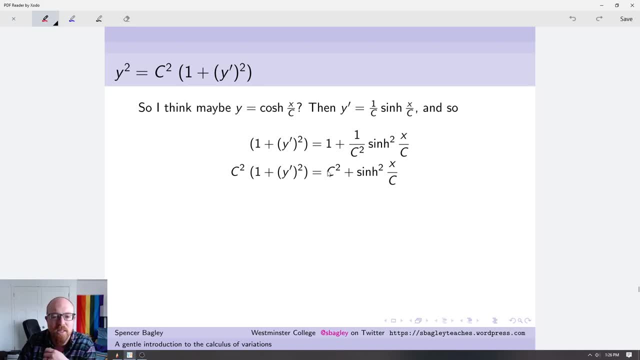 Uh, let's see if I multiply through by that c squared, Yeah, I've got a c squared plus this, which is not quite what I want. I would really like that to be a one, essentially, or this to be the same as some coefficient on. 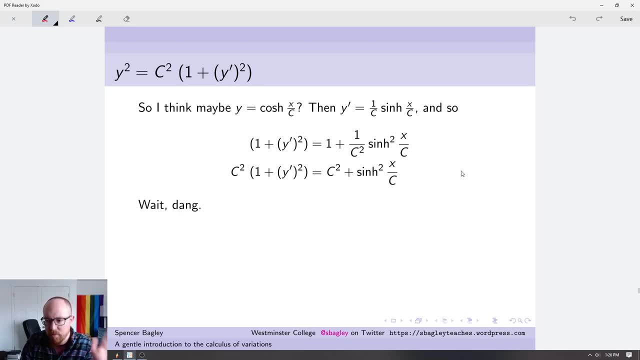 on my cinch squared. So I think that's probably the wrong guess. What if I modify my guess slightly? If I had a c here, then this would die. And so then, when I multiply by the c squared, I think I would get a c squared plus c squared. 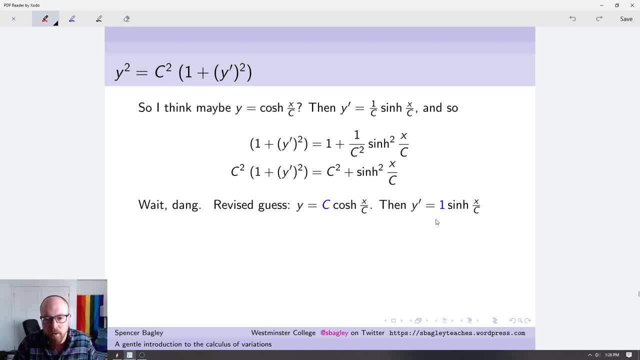 So here's my revised guess and let's see if that works. Um, yeah, okay, y prime now is one instead of one over c, times the cinch of x over c And uh, if I add one to that, um. 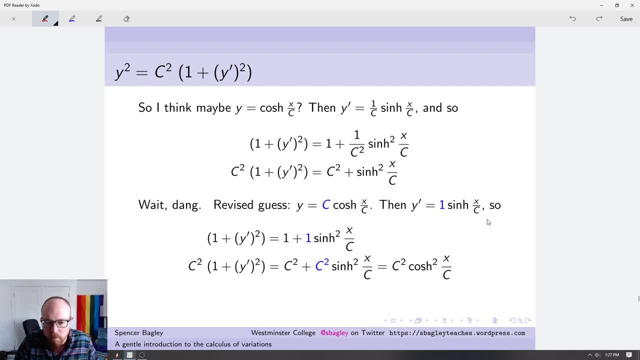 and then multiply by c squared, um, then I can do that Pythagorean thing and I get that is indeed y squared. So, um hooray, I have managed to guess the solution to this differential equation. um, by looking carefully at the structure and then knowing about the hyperbolic. 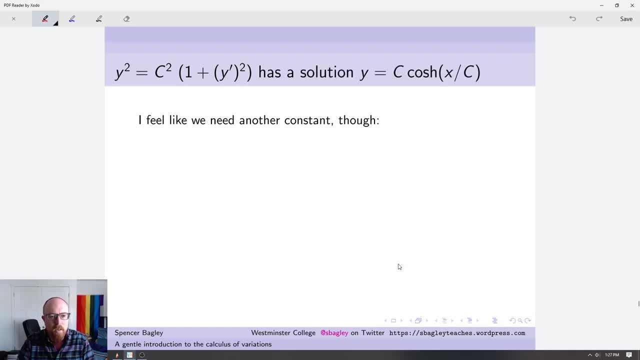 sign and hyperbolic cosine. Okay, this is cool. So I think that we have a solution. y equals c times the, the cosh of x over c. I don't think this is the general solution. I feel like we need another constant. 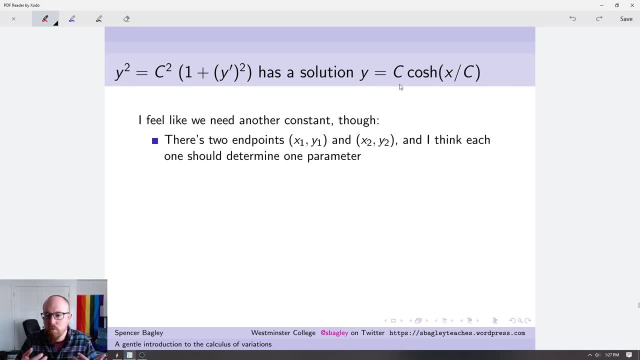 I have a constant, but there were several uh parameters right, There were several uh free choices that we had when we were setting up the problem, specifically the two end points. I could move any one of the end points around however I wanted. 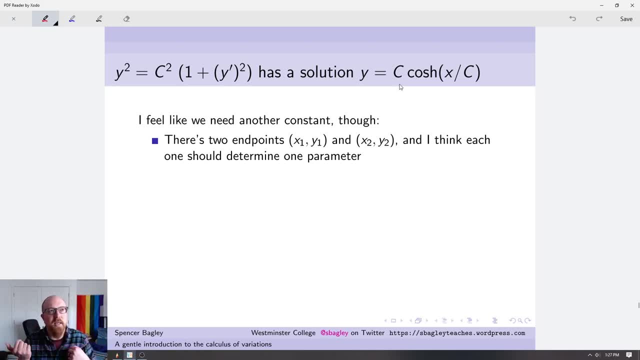 And so I feel like it, like my general heuristic, is that each free choice that I have ought to correspond in some way or help determine a one parameter. So, since I have these two free choices, I should probably have two parameters, Okay. 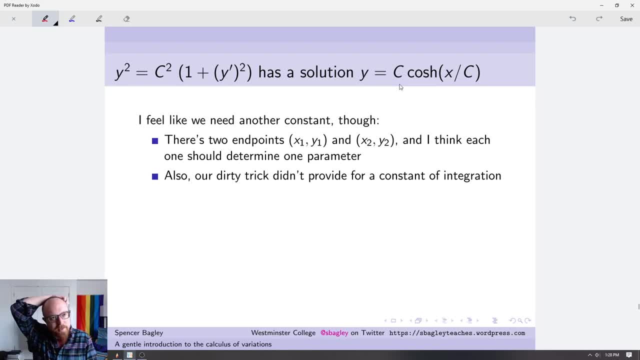 another thing that's that I'm noticing here is that that c that we had just came from, like the Beltrami identity, It was a constant of integration for something a long time ago. It wasn't a constant of integration for the, you know. 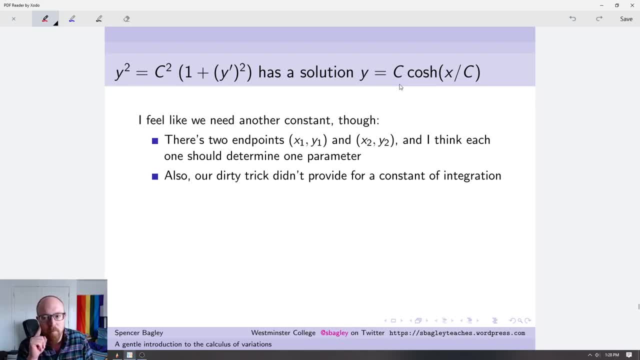 separable differential equation, right. So I think that I probably need like a constant of integration to to appear somewhere. Um? so here's another dirty trick. Notice that our differential equation was- was autonomous, right It was. it was invariant. 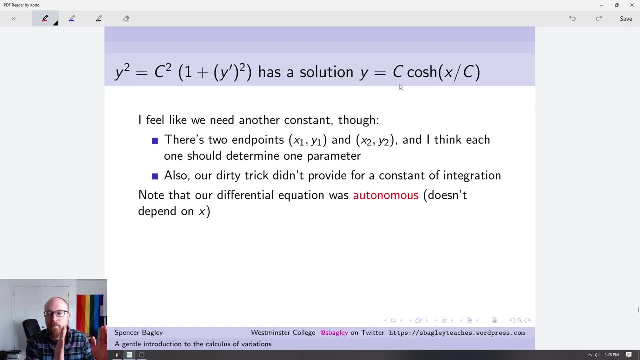 It doesn't depend on X And so it's invariant under horizontal shifts. And so probably, if I just replace X by like X minus H to allow for horizontal shifts, that's probably all I need, Um, and so I'm actually going to guess this and I'm going to let you pause and 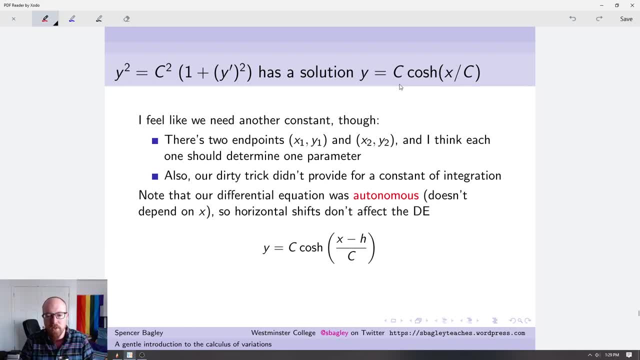 think for a second about how the calculation on the previous slide would change If there was an X minus H here. the answer is it kind of, doesn't Um, and so you can check that this. this will also satisfy this differential equation. 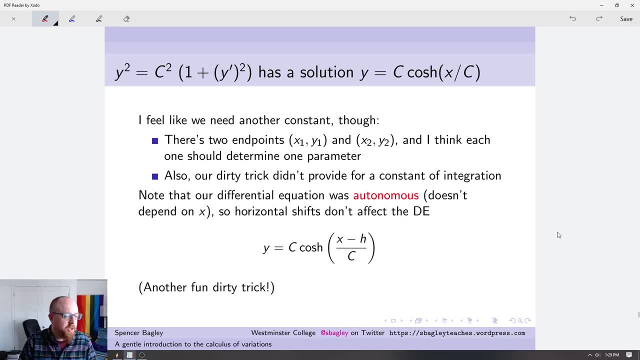 Um, this is another fun dirty trick. If your differential equation is autonomous and you don't know where your constant of integration is going to go, um see if just shifting the uh independent variable works. All right, There was. 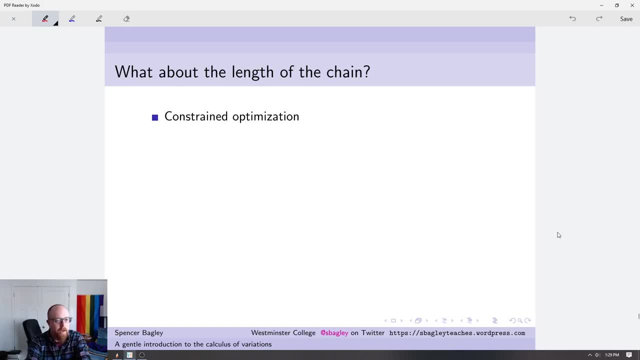 however, one more free choice that we had, which was the length of the chain, Um, and so we have landed. Therefore, since we haven't considered that so far, right, Um, if we consider the length of the chain, then we land in the situation of constrained optimization. 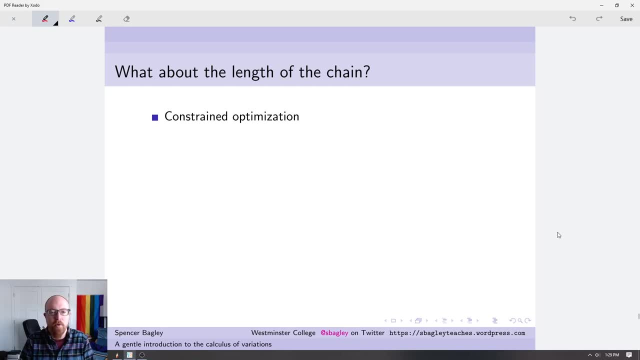 For those of you who have taken a multivariable calculus class. uh, you're having flashbacks to Lagrange multipliers. Yay, It's a little bit surprising that they appear again here. Um, here's how the Lagrange multiplier situation looks in multivariable calculus. 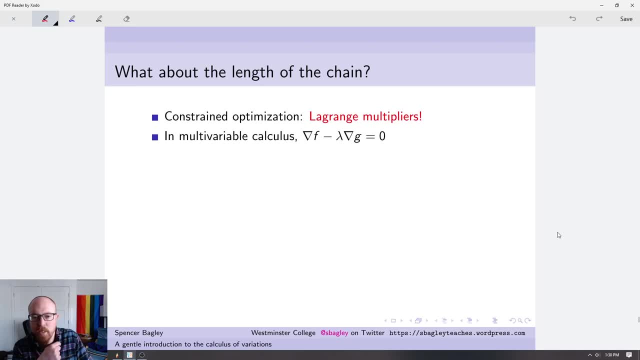 You've got. the gradient of F is supposed to be parallel to the gradient of G, right? So, uh, del F equals Lambda del G. subtract that over Um. this generalizes. Okay, I'm going to tell you right now that, for the next five minutes or so, 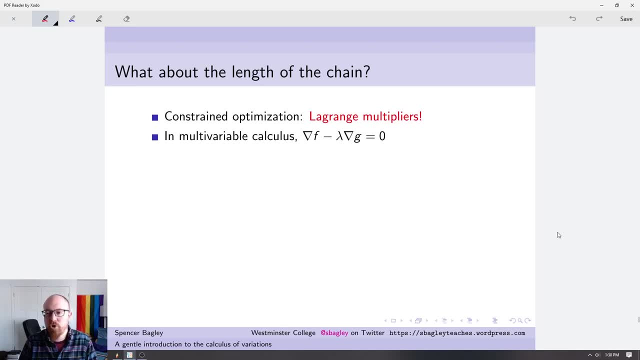 I want to give you a flavor of how this is going to work, And I'm going to be extremely imprecise and wave my hands a lot. Um, here's the first thing that I'm going to wave my hands about. I'm going to tell you that this generalizes. 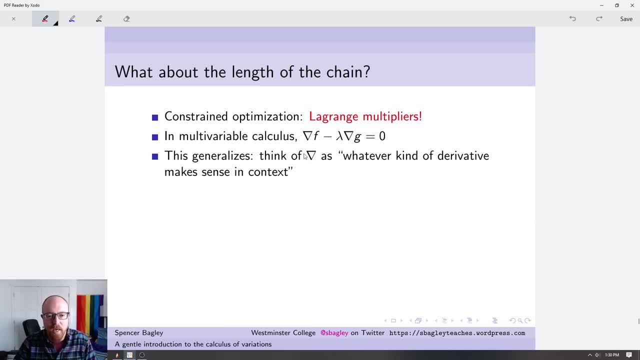 um, and you should just sort of think about of this sign as meaning whatever derivative it is that makes sense here. You can see I'm being extremely imprecise with this. Um, so our constraint is arc length and we know how to calculate the arc length. 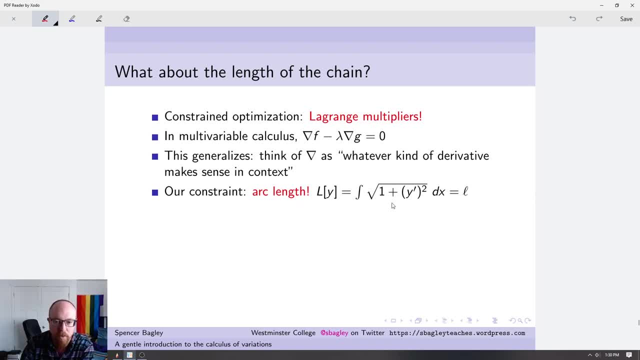 We did that a minute ago. Uh, we had some functional for that. We were integrating DS, and so we're saying that that equals some constant, which let's call it L? Um. okay, so that's our, that's our. 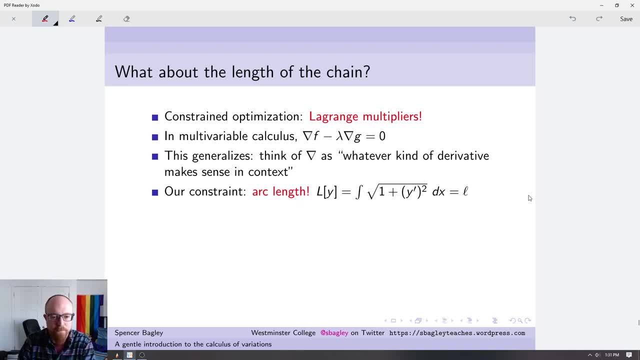 that's our G in the in the Lagrange multiplier situation. So if we set up right, uh, whatever kind of derivative makes sense, the function that we care about, optimizing Lambda for a Lagrange multiplier, whatever kind of derivative makes sense. 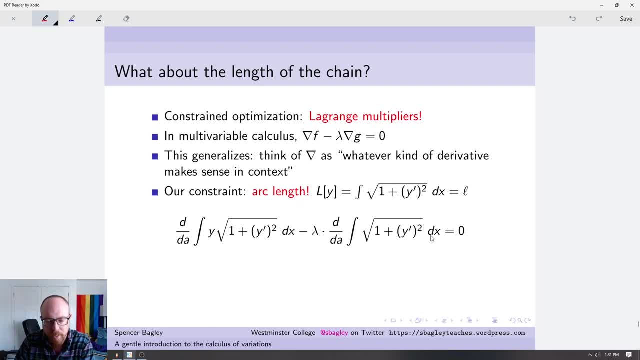 the function providing our constraint. Here's what this looks like. The derivative that we care about is the derivative with respect to a of you know, feeding a wiggle into the functional. I might- I maybe should- have written this with W's. 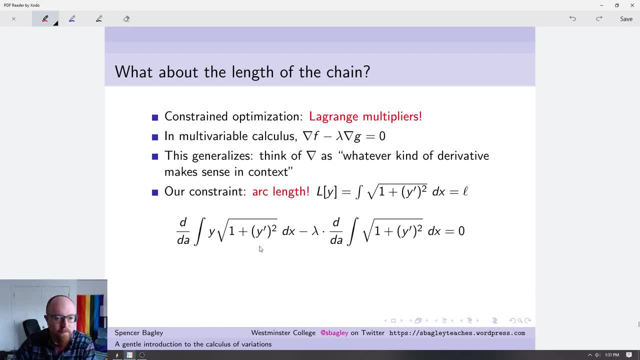 but that was confusing when I tried to write it down, So I didn't. So here's our derivative thing: that we're trying to optimize this. So this is our- uh, our GPE functional Lambda, the Lagrange multiplier, uh. 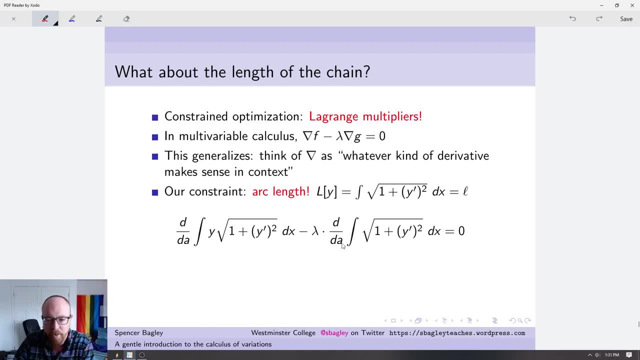 derivative that makes sense in context. uh, arc length functional. Okay, And then this is all supposed to equal zero. I'm going to use here the linearity of the derivative and the linearity of the definite integral to sort of smoosh some stuff together. 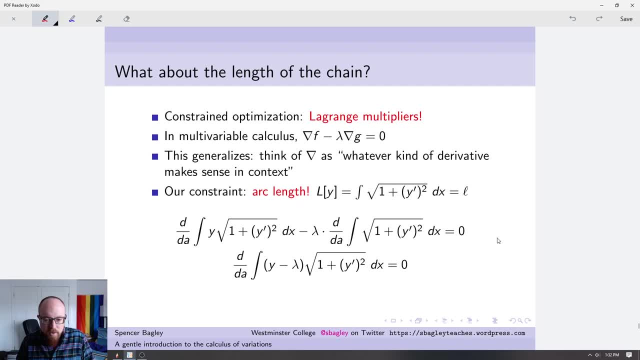 I think you will probably believe this is true. Um, and so this is cool. We have actually just landed in the original situation, but with a just slightly more complicated functional. uh, that is, a functional with a just slightly more complicated into grant. 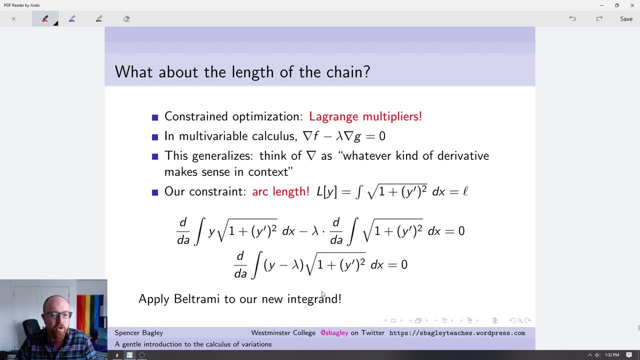 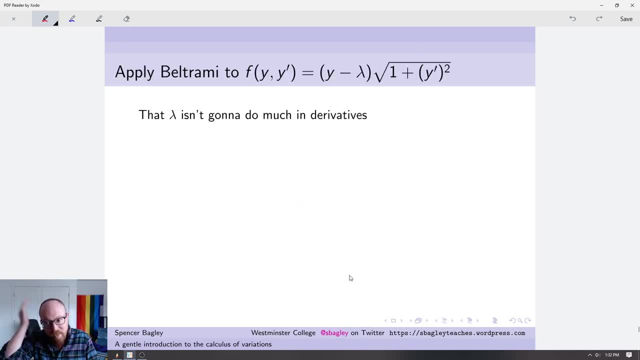 Um, so that means like we can just apply Beltrami to our new into grant. It still doesn't depend on X? Um, here's what this is going to look like. We basically already done it. That Lambda, that's here. 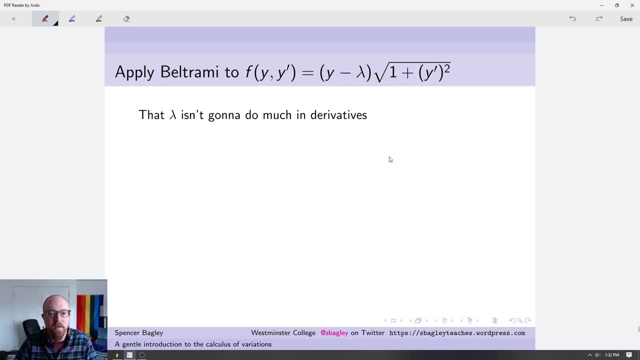 nothing. It isn't going to contribute in any way to any of the derivatives that we are doing. right, It's essentially just a vertical shift of the of the Y here and that doesn't really change much. Uh, so, and you can. 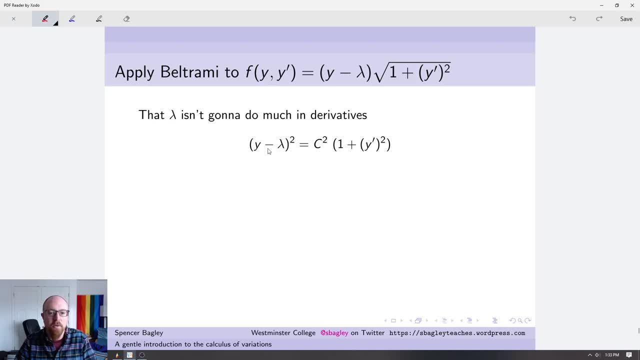 you know, work through, uh, but you'll find that the differential equation that you get is this, which is basically the same as the previous differential equation: Y squared equals blah, blah, blah. Okay, Um, and you can spot that this Y minus Lambda is just substituting for Y. 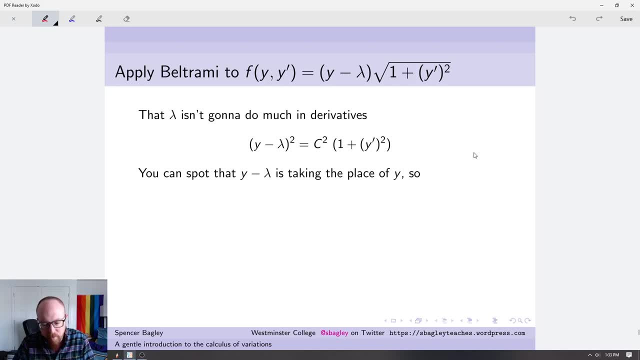 And so the solution to the differential equation will essentially be the same: Um, just Y, minus Lambda equals C, Koshan, uh, Kosh, blah, blah, blah. Add that Lambda over and here's what you get, And you can check that this works. 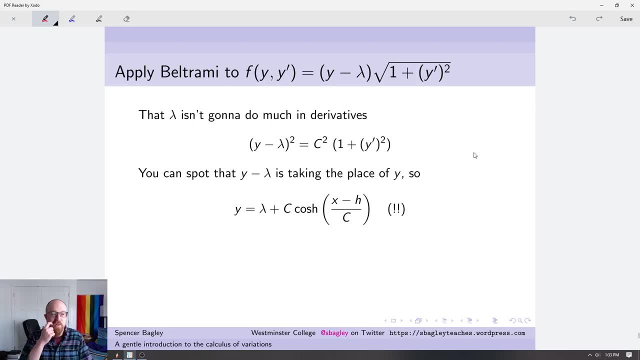 I promise, Uh, this is kind of remarkable that, um, figuring out how the length of the chain impacts things, just gave us one more parameter. That was just a vertical shift. It's kind of remarkable. Um, okay, now we have landed on something that has the correct number of parameters. 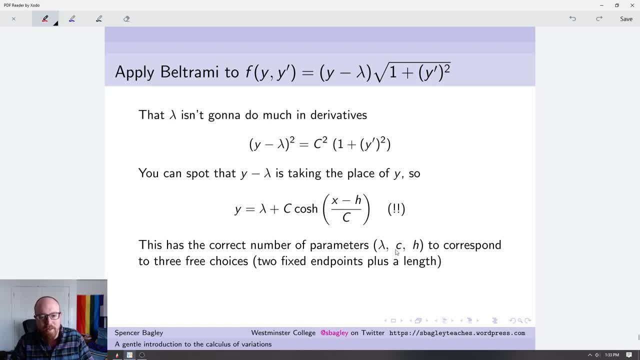 three Lambda, C and H. uh, that should be a capital C, Pretend it is Um, and that corresponds quite nicely with the three free choices that we have of the two fixed endpoints plus the length Um. in the small amount of time that we have left, 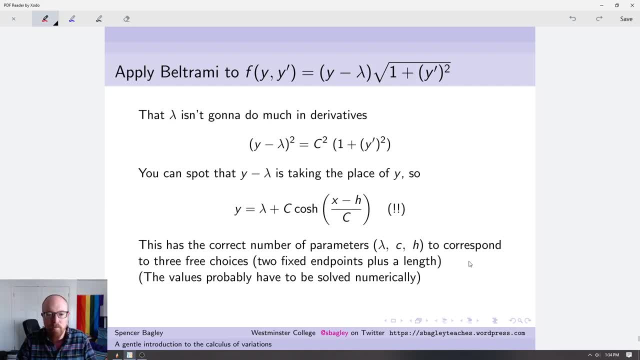 uh, I will just say that the values probably are going to have to be solved numerically. Um, that Kosh function is, uh, kind of a pain to work with. Um, but I I made this Desmos worksheet and I'm just going to show it to you.